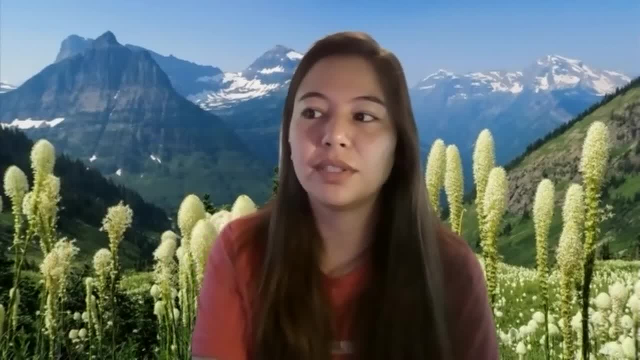 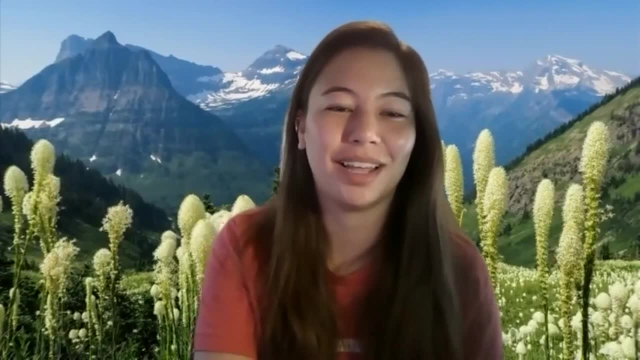 A proud UT alumnus, Ben completed his PhD at the University of Texas in 2019, Hookham, where he worked with Dr Charlie Cairns in his reservoir characterization research lab. If y'all just a few administrative things. if y'all could hold your questions till the end. 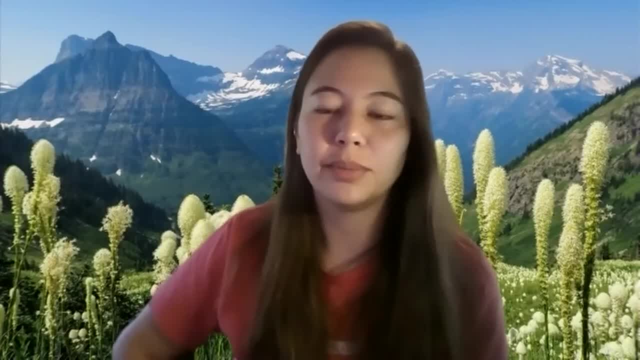 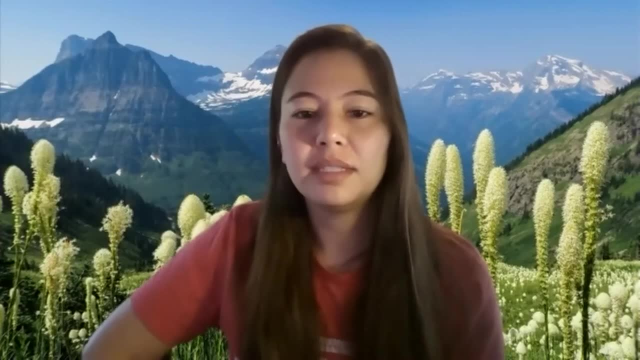 you're welcome to put them in the chat box, or, you know, at the end we can unmute ourselves and ask questions, but I would ask you not to ask questions during the talk, And this talk will be about 40 minutes and we'll do questions afterwards. Okay, Ben, rock and roll. 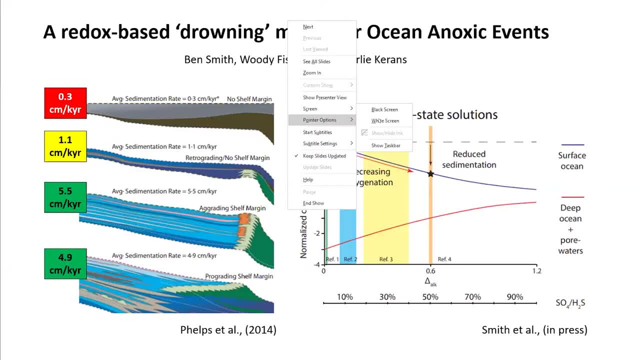 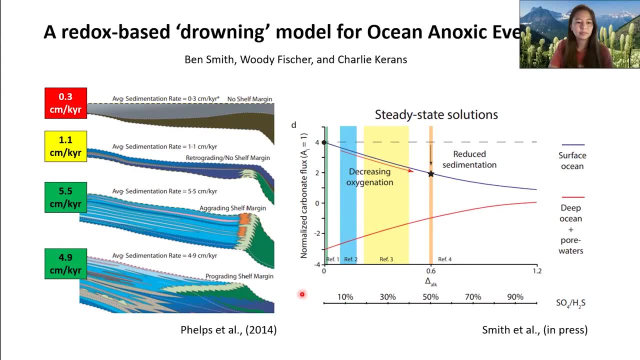 All right, let me just share my screen here. All right, how is that? Can everyone see that Yep looks good? All right, well, I'm really thrilled to be here today, and thank you for that introduction, Kelly. So yeah, my name is Ben Smith. I'm right now a postdoc at Caltech. 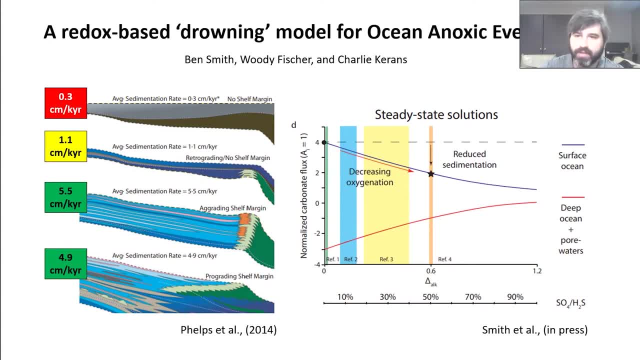 but I finished my PhD at UT in 2019, and there's actually a little bit of a personal story here, but the material that I'll be talking about today was something that I was introduced to very early on in my graduate career and then just really never touched in any significant way until 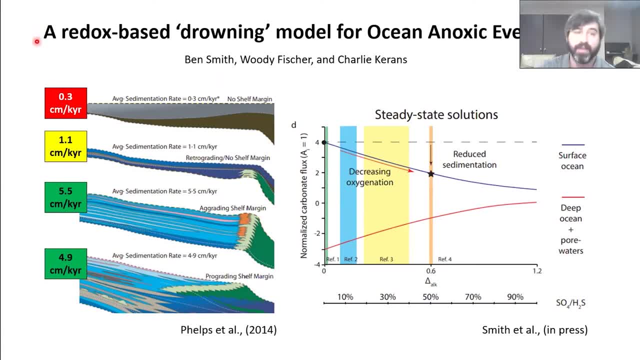 after I left UT, So it's been fun to kind of circle back to it. It'll be really fun to talk to everyone at the Bureau, because I was actually introduced to this through you know cores at the BEG core facility, and so I'd be really interested in getting the perspectives of you know people. 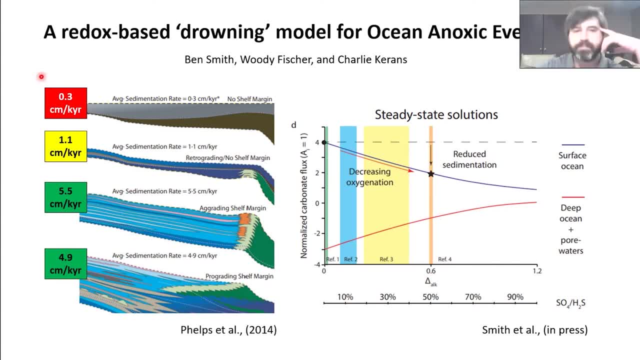 who still are working on those kinds of approaches. So the title of this work is A Redox-Based Drowning Model for Carbonated Platforms During Ocean Anoxic Events. So I'm going to start by kind of explaining what some of those words are. 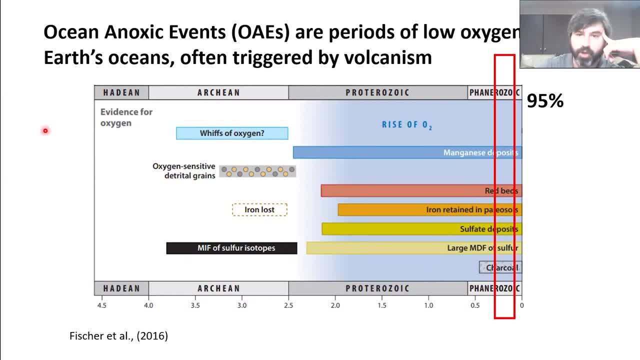 and I'm going to start with that kind of big picture Earth history perspective, which is that, you know, oxygen in today's world is ubiquitous. It's one of the most common gases in the atmosphere and about 95 percent of seawater has oxygen, all the way up to the ocean. So it's a 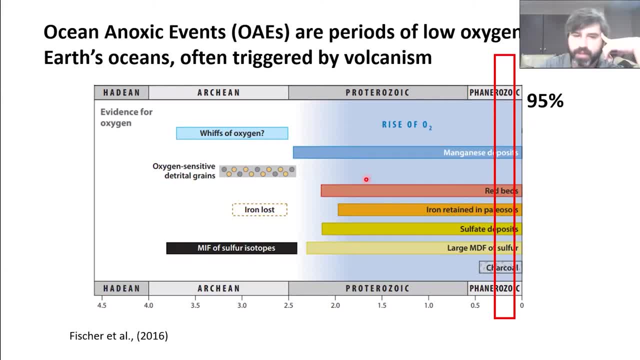 ocean floor. The Earth historian's view is that this is, you know, a relatively recent state of affairs. Oxygen probably first started accumulating around, you know, 2.1 billion years ago in Earth's atmosphere, and then it was probably wasn't until just before the Phanerozoic that we started. 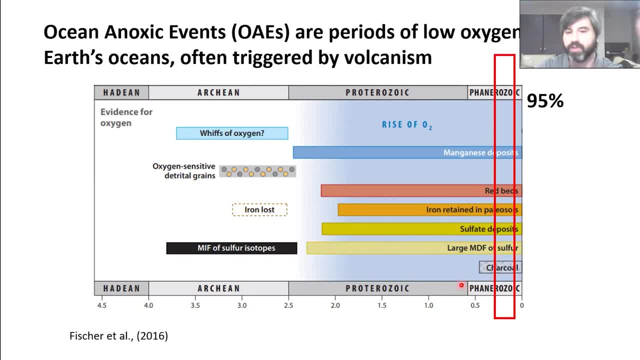 getting a lot of oxygen all the way to the bottom of the ocean, And so an ocean anoxic event is really a short-term reversal in this trend. The long-term trend is one of increasing oxygen in Earth's atmospheres and oceans, and there's 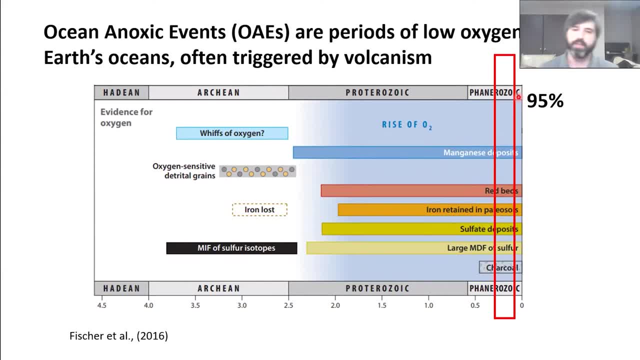 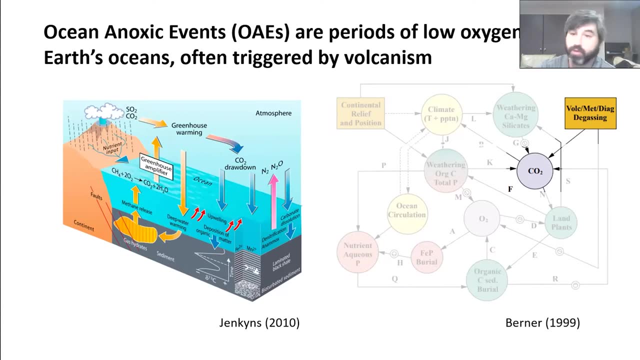 brief periods in the Phanerozoic where this trend reverses And we never really go all the way back to the world of the Precambrian. but it is this kind of interesting reversal And these reversals have a lot of important implications both for academic research and for petroleum systems. and 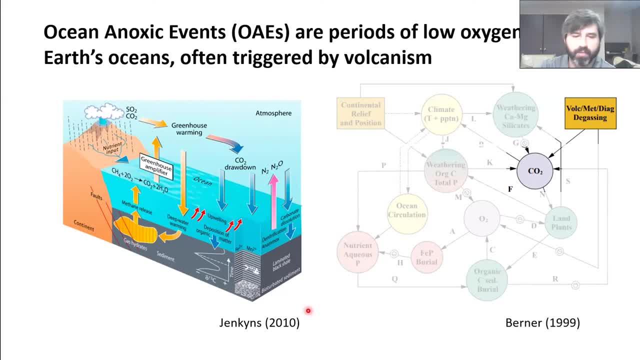 applied research. So like a classic review paper or a set of models, will probably look something like a little sketch. These events are usually triggered by volcanism. There's a kind of an outgassing of volatiles like CO2 and sulfur species, And then there's just a bunch of arrows that show. 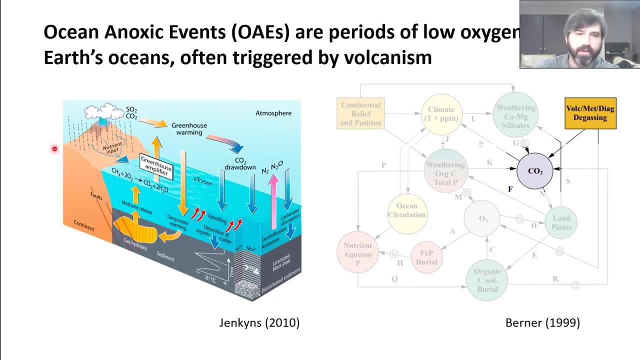 exchange between the atmosphere and the oceans and Earth's weathering feedbacks, And so a lot of times you'll see this drawn as kind of this web or diagram where you have this volcanic eruption of CO2, and then there's this cascade of feedbacks. 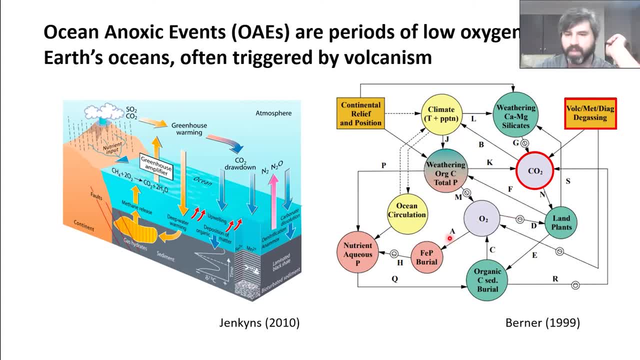 You can trace all the arrows through these little boxes, but it's complicated And one of the reasons people are really interested in this is because it touches on almost every important Earth surface processor system. Touches on climate weathering, feedbacks between burial of organic matter and 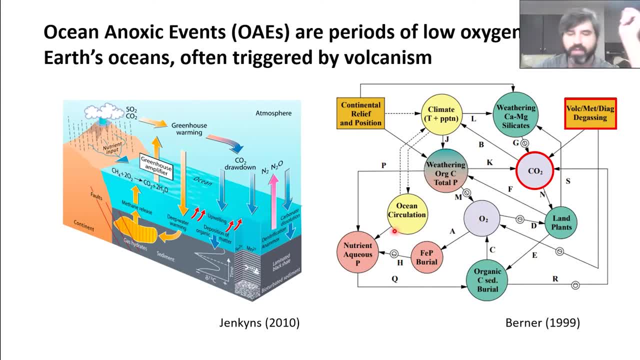 Earth's redox species- And I think that's part of the promise of why we study these events- is if we can understand what's going on in ocean anoxic events. that indicates we have a pretty good understanding of how these systems are linked And that has added a lot of value to 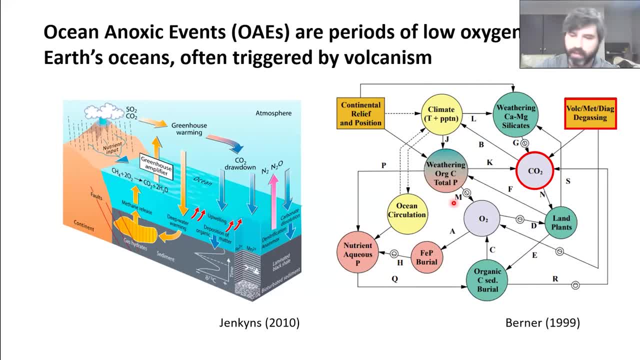 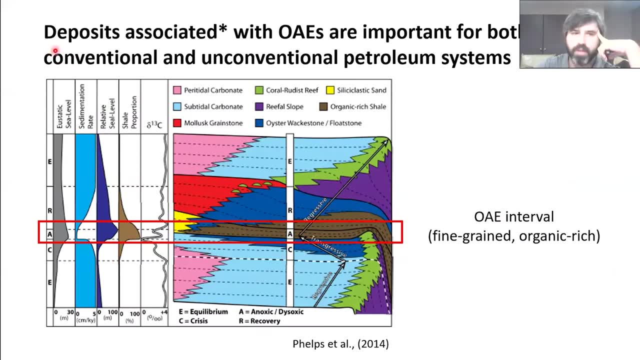 applications both for modern climate research and for understanding the habitability of our planet in deep time. There's also a kind of an applied perspective because a lot of these deposits are important for both conventional and unconventional petroleum systems And I know that's a big focus of a lot of the research groups at the BEG and that's actually how I was introduced. 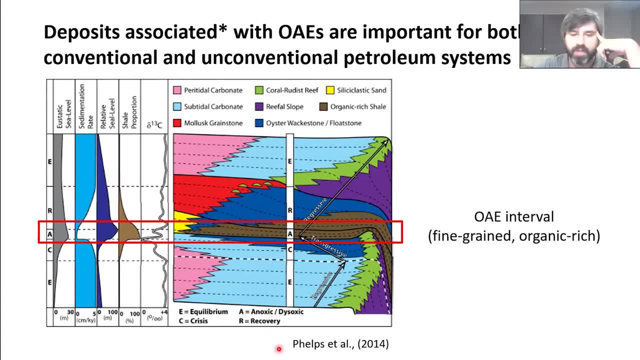 to the problem as well. So this diagram here is kind of a summary diagram from another PhD student at UT And he was really interested in kind of shallow water carbonate systems and how they respond to these ocean anoxic events And so kind of the classic signature in these carbonate. 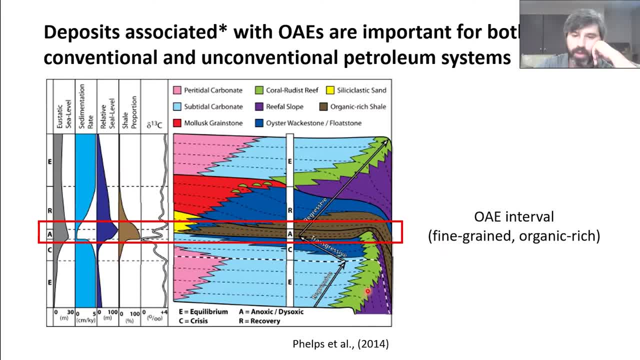 environments is that, during an ocean anoxic event, we're going to replace some of these shallow water carbonates with fine-grained organic rich deposits, And that should somehow correlate with the geochemical changes that are indicative of this web of persistent feedbacks. 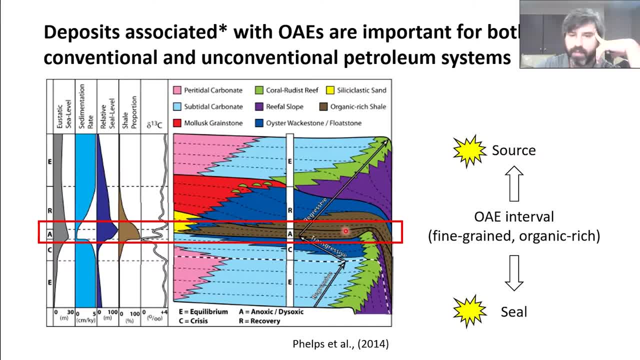 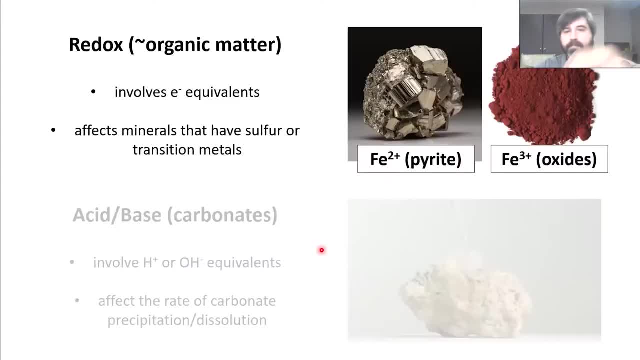 And these organic rich deposits. in the context of a conventional petroleum system, they could be a source for petroleum or they could seal underlying carbonate reservoirs, And then just kind of a little bit of background. it's like, okay, so we've got this web of feedbacks of surface processes, but what we're usually left with is: 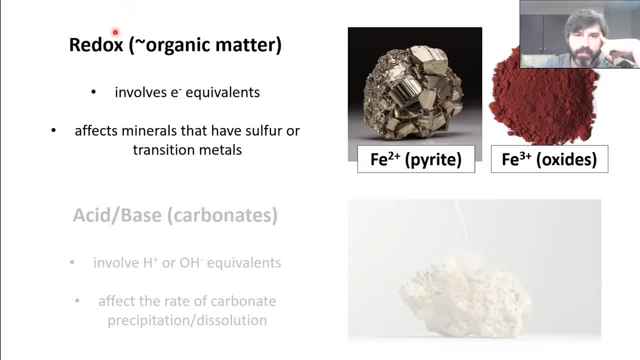 a series of sedimentary rocks, And so part of this game is trying to figure out what we can pull out of the rock record and how it has to do with these processes. And when it comes to this, when it comes to organic matter burial, most people are interested in redox, the change of 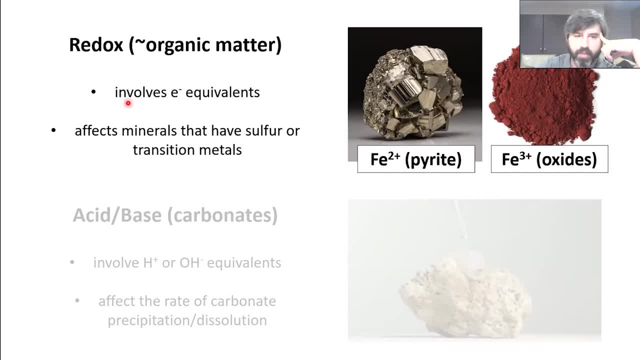 redox species within Earth's oceans, And so just kind of remember that that involves electron equivalence and it usually involves something like sulfur or transition metals that can have multiple valence states, And the way we do that is when the valence state of these 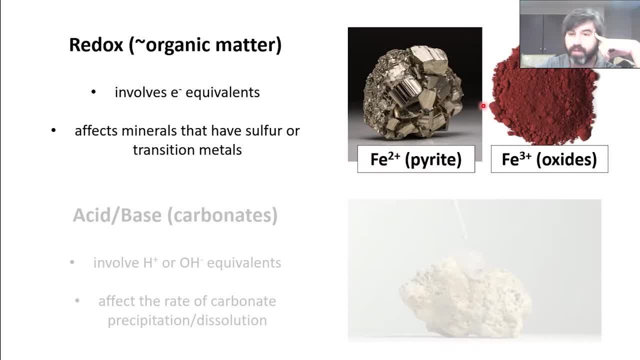 atoms changes, it'll slot into different minerals and those minerals have different solubility. So someone like Todi Larsen will work with technique like x-ray fluorescence and it'll kind of look for changes in these trace elements that are correlated with changes in mineralogy and by proxy changes in redox. 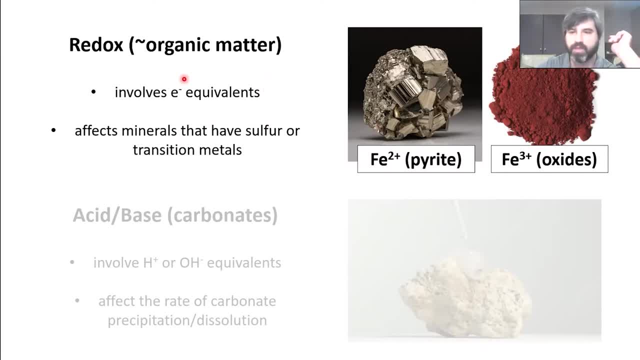 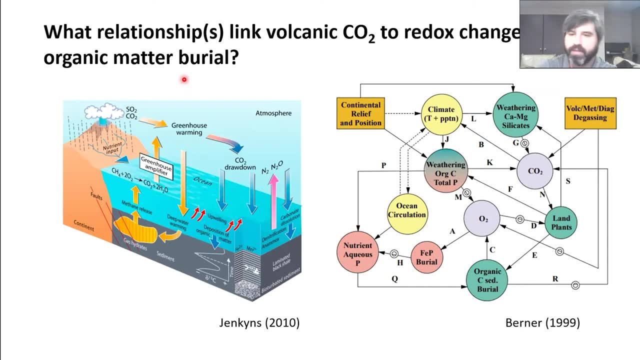 And so that's a huge part of these events, and it's usually related to organic matter: Abendor Hunt kommen, Thomas Daubnermüller, MD. And then kind of return to this diagram. this kind of again highlights how length these systems are, which is like 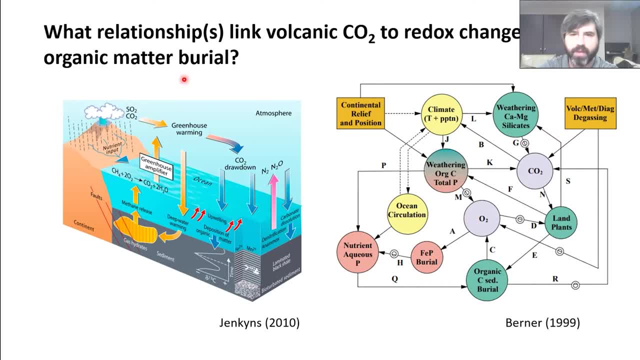 okay, what's the pathway that connects redox changes and organic matter burial to this kind of co2 volcanism story? um, it's actually really complicated and if i was to trace a path on one of these kind of summary web figures, it would be like: okay, i inject a bunch of co2 in. 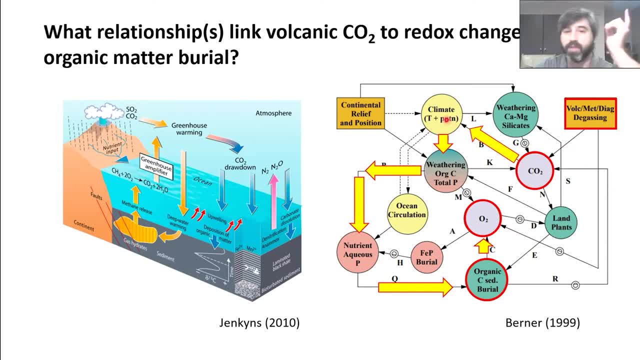 the atmosphere. that changes earth's climate system, including its temperature and precipitation. that changes the weathering on the continents. that brings a lot of nutrients into the ocean, which triggers a bunch of primary production of organic material. some of that organic material is buried and then, in an effort to consume that material, microbes exhaust oxygen in the ocean. 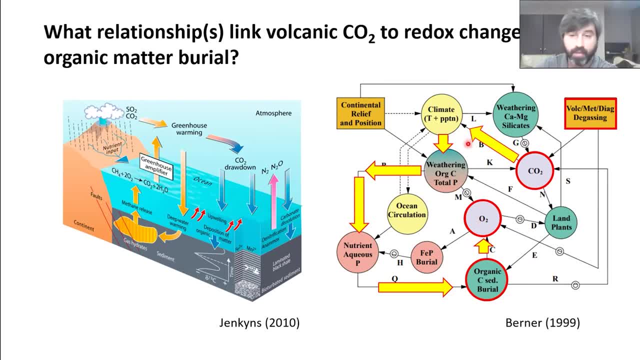 and so that's really, really complicated and you could spend, you know, a lot of time trying to work out the individual parts of these pathways and you also get a sense that this is a little bit of a multiple choice history. i could have maybe traced a different path, and so part of the 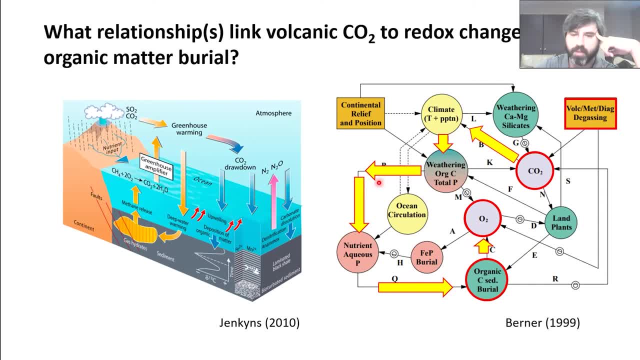 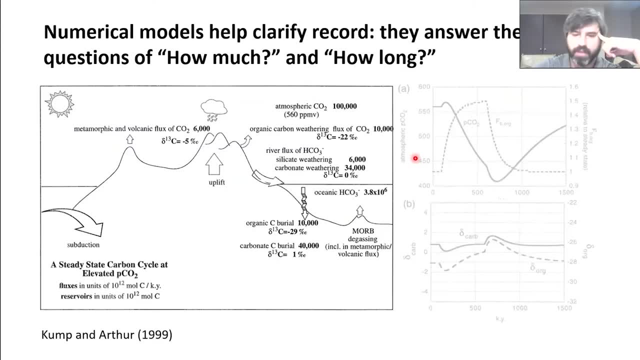 challenge is: you know, okay, which of these, you know pathways, are the most important? um, how do i judge between pathways? and then there's also this geologic perspective of you know. that diagram doesn't really give me a sense of time or of how strong those processes are. 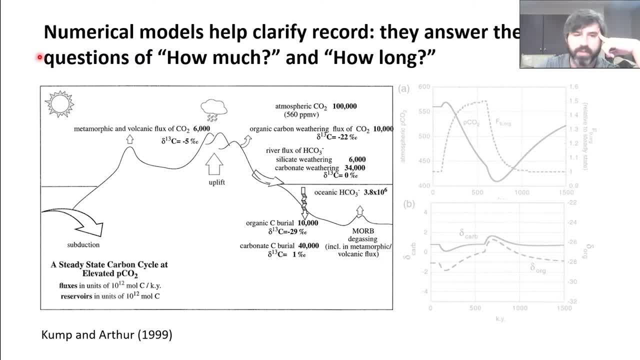 and so usually there's. there's other approaches that we use to fill in some of this information, and the one we'll be talking about today is numerical box modeling, and so the the way these box models are set up is they're almost like a toy. um uh, that kind of shows how the earth system. 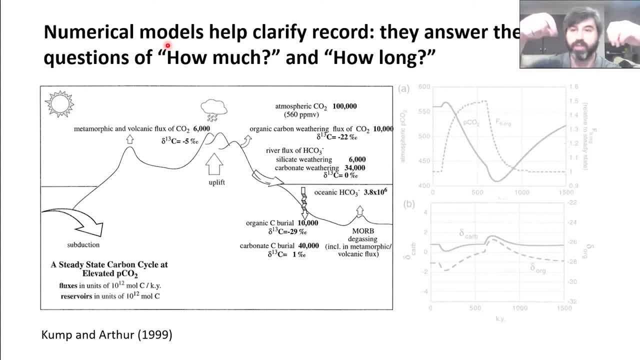 responds to changes, and so i kind of think of it like a guitar string. you pluck the guitar string and then the vibrations kind of ripple out, and so the ways are usually set up is: you have a, a set of fluxes and you want to transform. you want to somehow transform those. 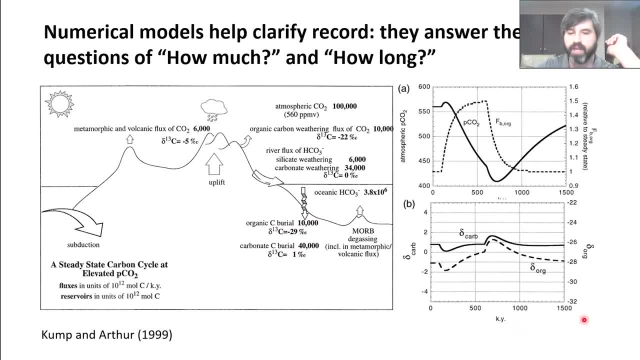 um into these, these plots that have time on one axis and then some something that's measurable within the stratigraphic record on another axis. so this is, um an excerpt from a famous set of studies from penn state, and and they, what they've done is they've taken this atmospheric pco2 as 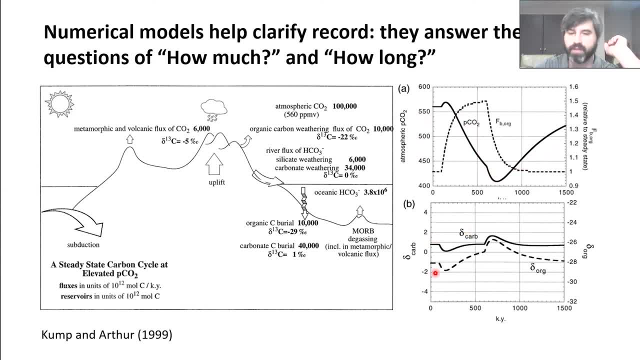 their input and they're using this link system to describe. you know, if i perturb atmosphere, co2, how is that going to affect carbon isotopes in carbonates in organic matter? because those are two things i can measure in the rock record, and so the way i think of this is numerical. 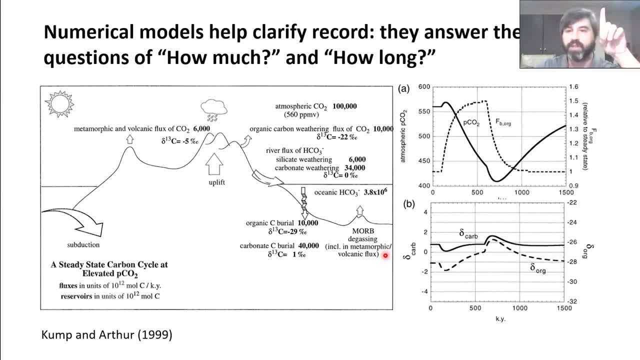 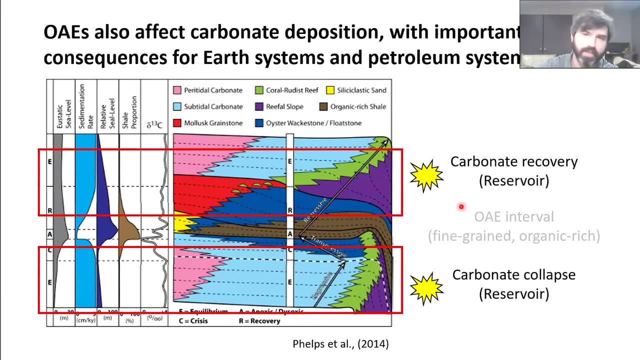 models give me a sense of how much, and then they give me a sense of how long. you know what kind of time scales do these processes operate over, and can i match that to the time scale that i'm seeing the stratigraphic record, and so i would say the majority of oae. what oae is the acronym for these? 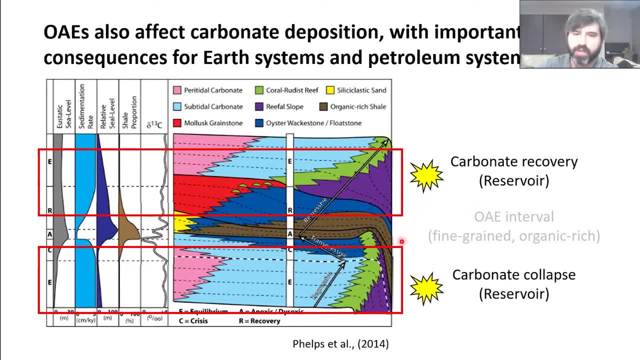 majority of oae research is has really been focused on the organic matter side of it, but there's this other part of the story: in these shallow water carbonated environments, and that the carbonate system is also affected, um, and that's what i want to talk about today. 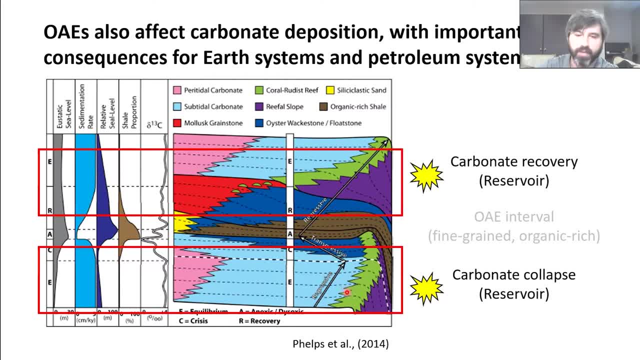 and specifically i want to talk about this, this pattern where, just prior to this, these uh fine grain deposits kind of being deposited on top of these platforms, there's usually this pattern of backstepping and drowning, and this is usually sometimes called carbonate collapse or or um platform drowning, and this was really first outlined in a series of kind of seminal. 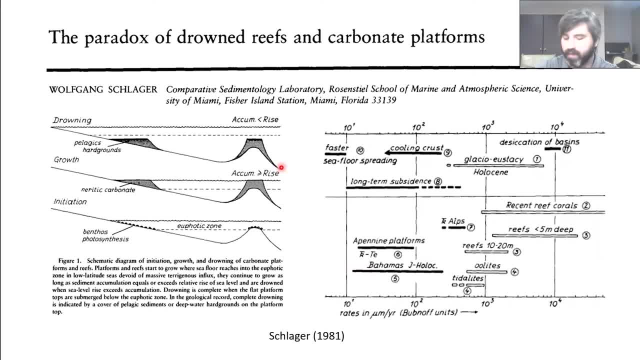 papers in the 80s and this was kind of the height of uh one sequence- stratigraphy was kind of first coming into its kind of kind of coming into its own as a discipline. and there's a paper by uh, wolfgang schlager where he outlines what he calls the paradox of drowned reefs and platforms. um and 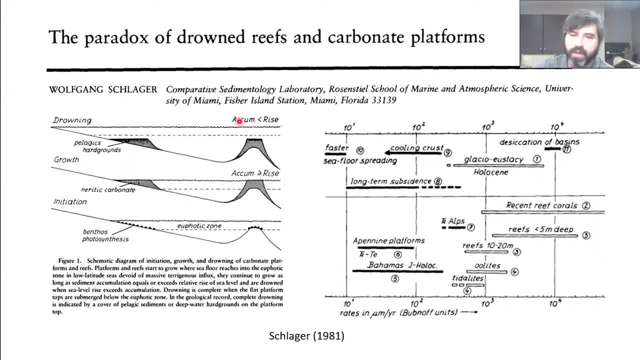 schlager was uh was working in miami. he was doing a lot of work on modern carbonate systems and he's been doing a lot of work on sedimentation rates and plasticine carbonate systems both in great bahama bank and florida and he had kind of done some work measuring sedimentation rates in these. 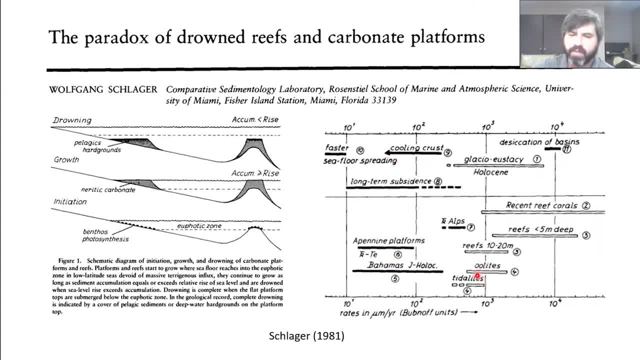 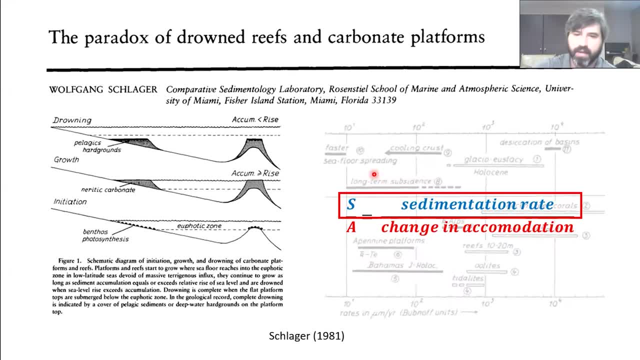 environments. and he ran into this problem where, if he measured sedimentation rates, either in modern platforms or in ancient platforms, and he tried to balance that, um, when he tried to balance that against the rate at which new space was being created for sediments, he, in his opinion, the 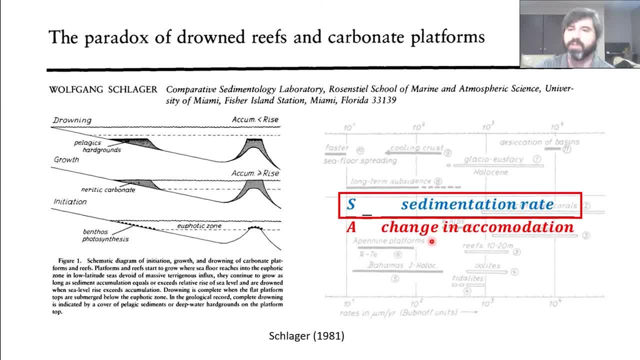 sedimentation rates were so high that would be very, very difficult to generate these backstepping through things like subsidence, tectonics or sea level change, and so he he suggested that maybe, uh, the solution for some of these drowning events was to play with the sedimentation rate. 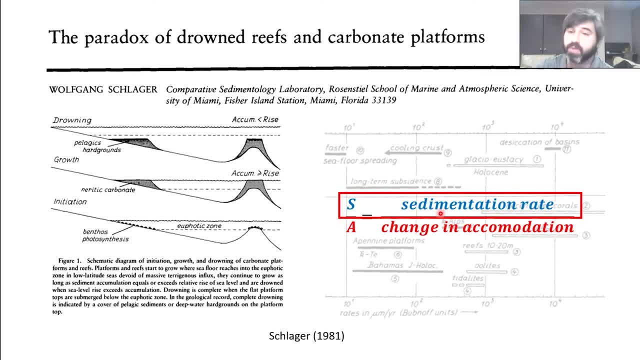 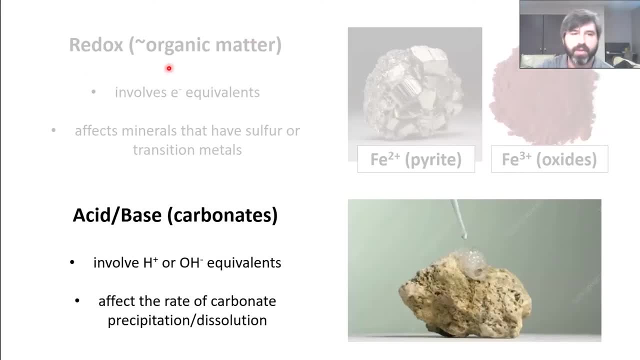 and to look for feedbacks that would damage the way that carbonate is precipitated in the ocean, um, and and so that kind of brings us to the second aspect of this, which is, you know, a lot of the uh research into oaes has been on the kind of redox side of things, but there's also this acid. 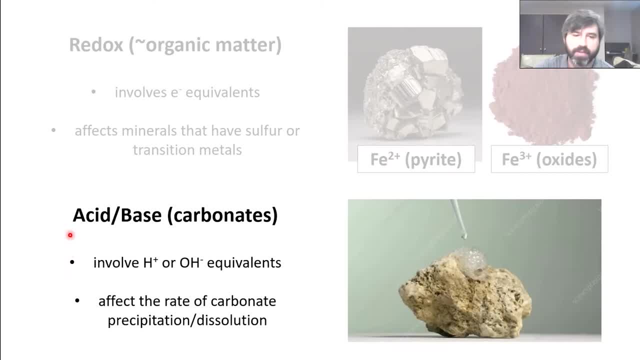 chemistry of seawater, which is very difficult, uh, to work with geologically because there aren't really good ph proxies, but it's, it's important for for carbonates and if you, if you're not um, if you're not well versed in chemistry or you kind of don't remember your um, your kind of geology, 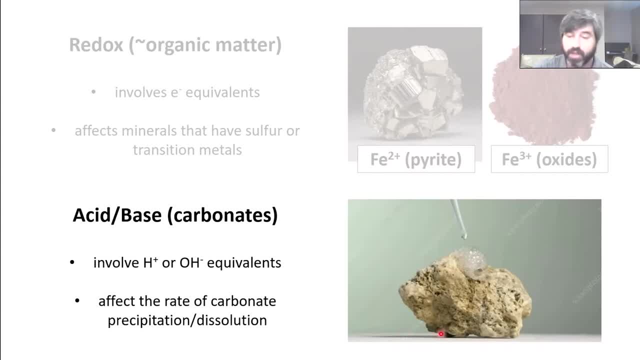 classes. the way i think of this is: you know if you have an introductory uh lab or field geology course? uh, one of the first, one of the things i'll ask you to do is i'll ask you to identify some of the things that you're interested in, and then i'll ask you to identify some of the things. 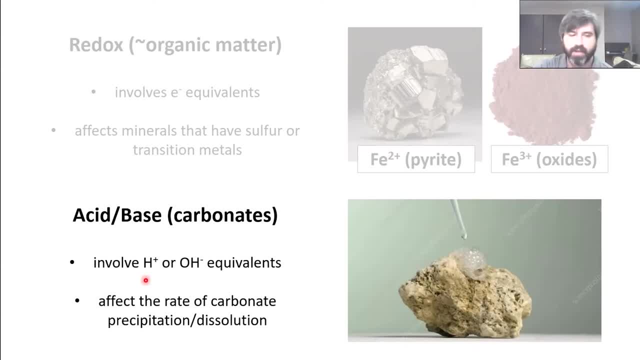 that you're interested in, and then i'll ask you to identify some of the things that you don't, and the typical way you do that is you'll drop a little bit of dilute hcl on that, and so so, if you can remember for the rest of the talk that, uh, you know, you know, dropping acid uh is bad for. 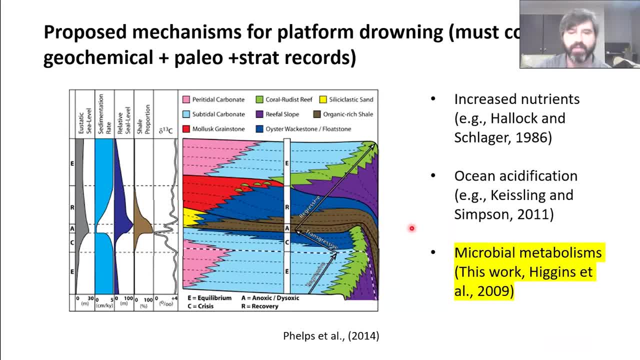 carbonates, then you know, we'll be able to get through some of the chemistry in this talk. and so that kind of brings us again to this, this idea of a multiple choice history which is: you know what? are you know in that kind of complicated web diagram, which of those arms or feedback loops? 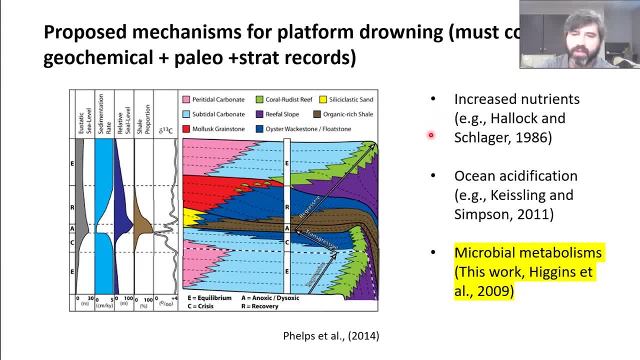 could reasonably damage the carbonate system, and i think there's at least three, three proposed mechanisms. one has to do with uh, nutrient poisoning, which i think unfortunately we won't talk about today. but the other two i want to talk about are ocean acidification and then kind of a 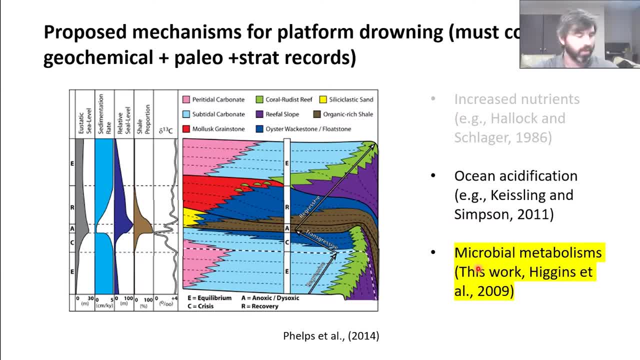 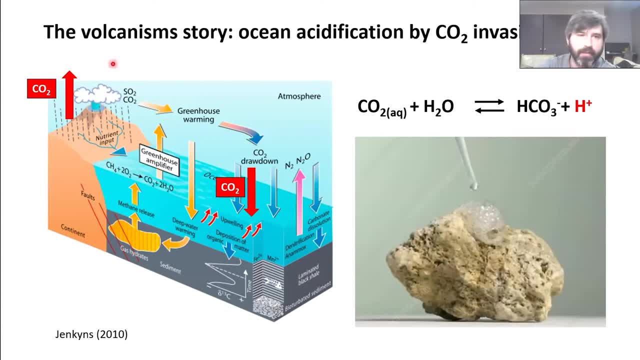 mechanism based on microbial metabolisms, which is, you know, what we've proposed in this work. so let's start with ocean acidification. um, this, this has been a really popular hypothesis for past 15 years and again it speaks to the interdisciplinary nature of this research, because a lot of these concepts have been borrowed from modern climate change literature. 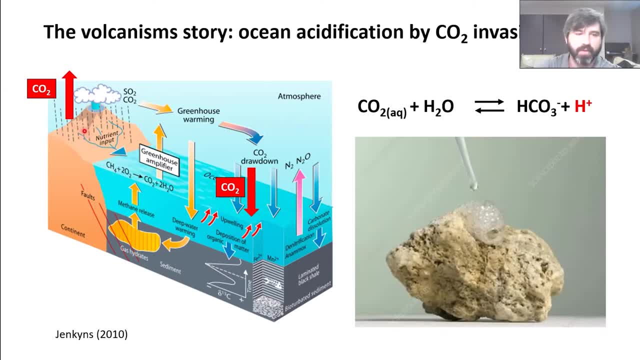 i think what people do is they look at this. they say, oh okay, well, the volcanoes release co2, and rapid co2 injection is also, you know, going on in today's world. so what are the kind of feedbacks that will happen? and so if you open up a news article about ocean acidification, it's going to 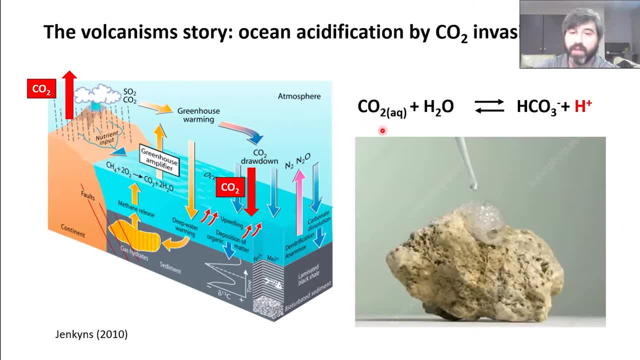 look something like this. so the first thing that's going to happen is that the ocean acidification will react with a carbonate molecule, which is that co2 acts as a weak acid in water. so co2 that's injected in the atmosphere will make its way into the surface ocean. it'll react with a water molecule. it'll. 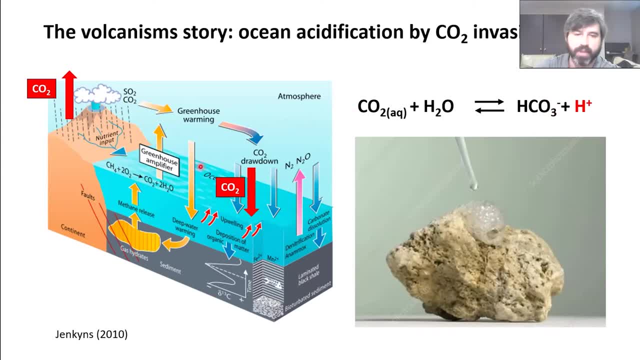 produce another carbonate species and a proton, and so that's like, on the surface, that's actually. that's pretty straightforward. it gives me a very direct connection between the, the underlying trigger for these events, and the stratigraphic record, and so i just want to point out this will: 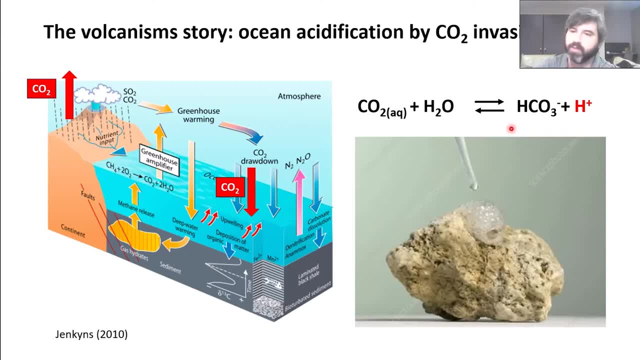 be a little bit more general, but usually what will happen is this will slow the rate at which carbonates are precipitated. so, from the perspective of platform drowning, if i'm slowing the the precipitation rate that actually may produce this kind of backstepping pattern, because i 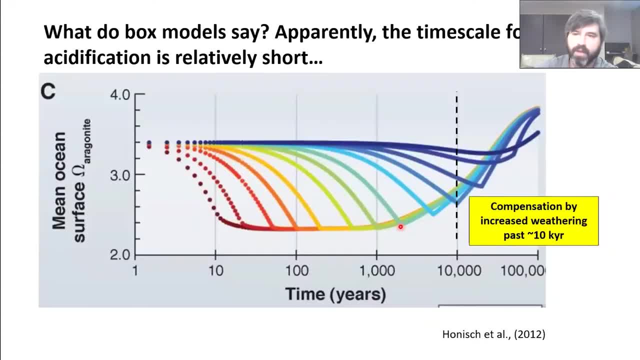 can no longer keep up with the background substance: great. so that's kind of the qualitative understanding. so so again, i want to turn to this tool of box modeling, which is usually the next step, which is all right. i want to use a box model to answer two questions, which is like: how long? 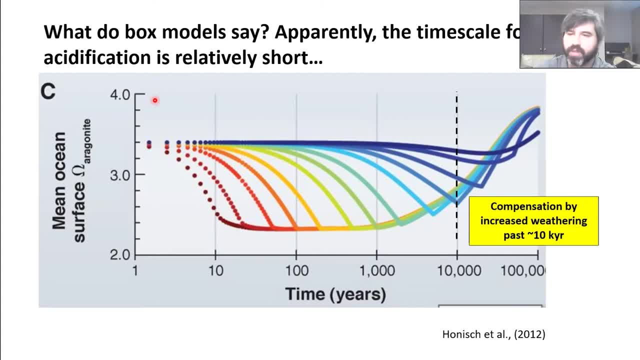 and how much. And this is where I think I start to run into problems with this ocean acidification mechanism. So this is from a paper in 2012.. It's a series of box model outputs The horizontal axis. here is time, And I want to point out that this is a log scale. So this is 10 years, 100 years. 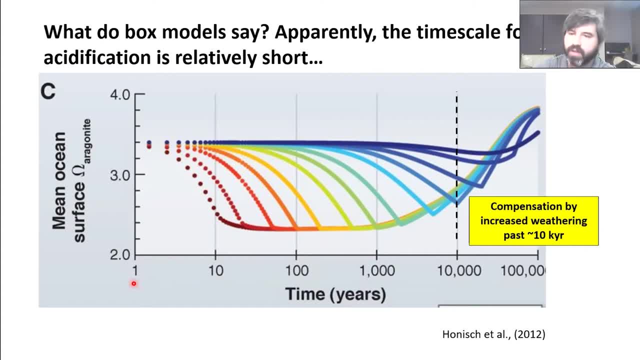 So this is about the human time scales that are usually considered in climate change research, And then, once we get up to here, 10,000, 100,000 years- a million years, which is very relevant for stratigraphic research- is going to be off this plot, But there's kind of this issue of time. 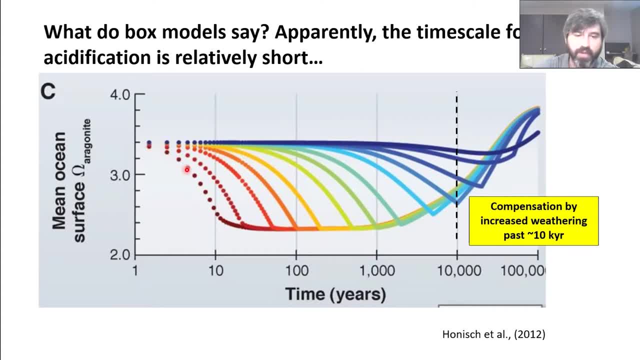 scale, And so the way this model works is that they double the atmospheric CO2.. And then they're using this capital Greek letter, omega, which is a measure of how favorable or unfavorable carbonate precipitation is in the ocean, And they're seeing how the surface ocean responds to this change. 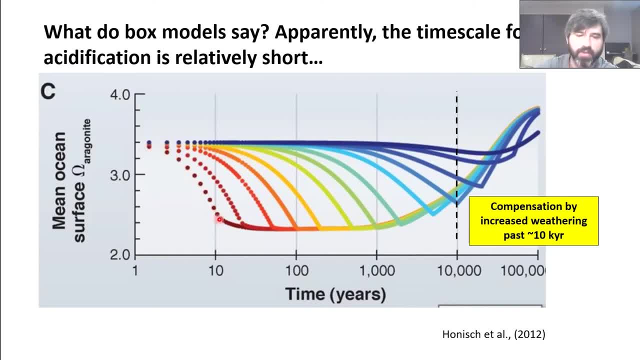 And so in the red models here they're doubling CO2 very, very quickly, over 10 years or so, And in the blue model they're doubling CO2 at a much slower rate. And in all cases there are other feedbacks within that web that start to push the ocean back to its starting. 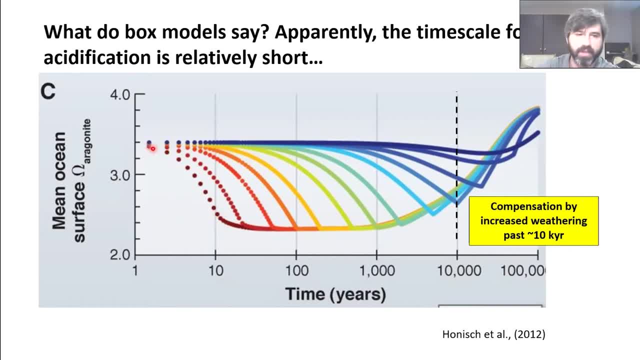 condition And the kind of thing about this is: you know I can damage the carbonate system by injecting a lot of CO2 very quickly, But that means the time scale of recovery is also going to be fast, at least geologically, And by the time I'm getting out to about 10,000 years, I've- actually I'm- well on my way to. 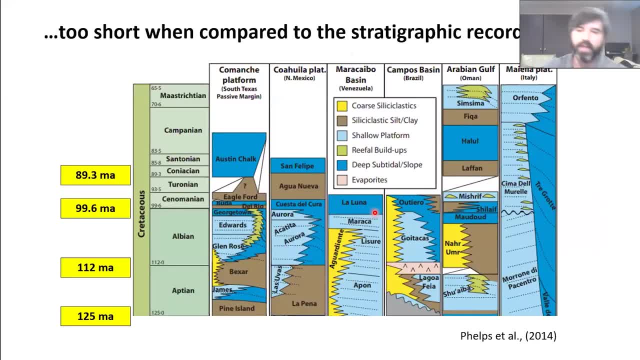 restoring the ocean to its starting state, And that's actually a really big problem for me. And again, this is PhD work that was done at the University of Texas. This is called a Wheeler diagram. The horizontal axis here is not thickness, but it's in time, And this shows the kind of the 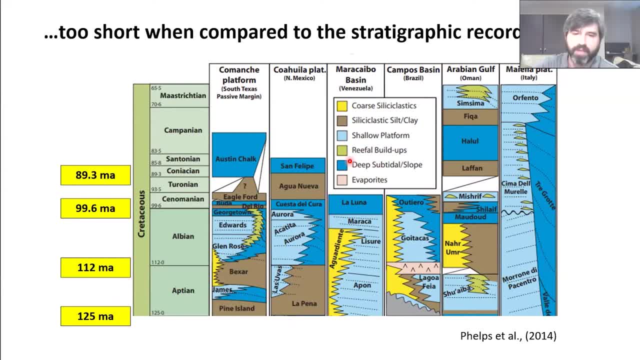 ages and times associated with some of these platform drowning events. And again here, the brown is usually fine grain material, probably organic, rich, And you can see that you know a lot of these are on the scale of millions of years, you know, probably a million years or 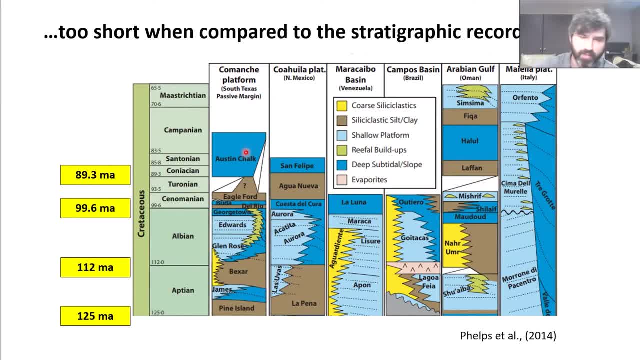 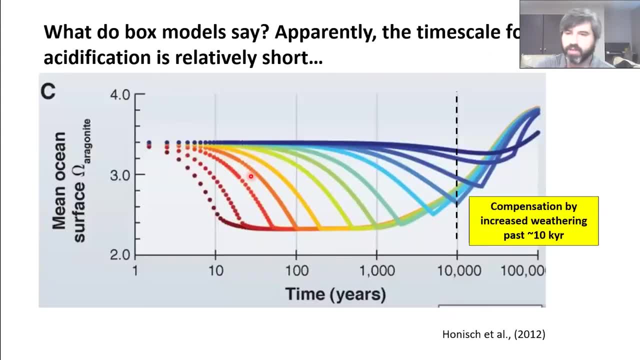 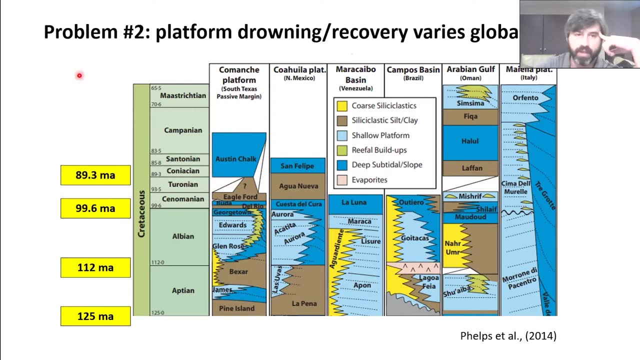 5 million years, And I always had this problem with this because you know that's too long for the time scale of ocean acidification that's suggested by a lot of these box models. Okay, there's also a secondary problem with this, which is that ocean acidification is a very 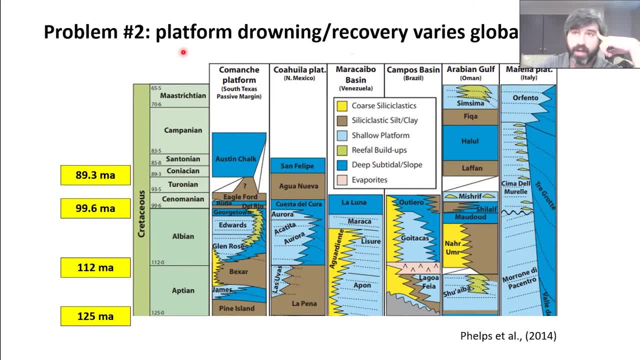 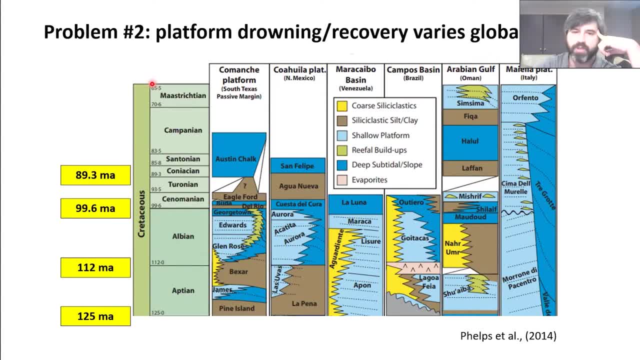 geochemical record, And what I mean by that is the atmosphere and oceans tend to be very well mixed with respect to carbon on kind of hundreds of years and 1000s of year time scales, And so one of the things that jumps out about to me about this diagram is a lot of these drowning events. 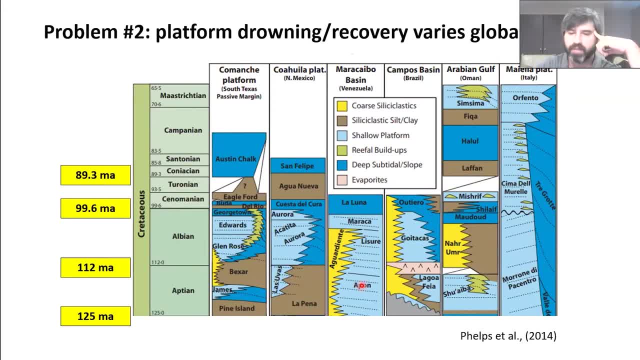 are not correlative with each other. You know the onset might be delayed or there might be, you know, areas, like in Italy, where we don't actually see drowning in the sense of these fine grain deposits making their way up onto the platform. 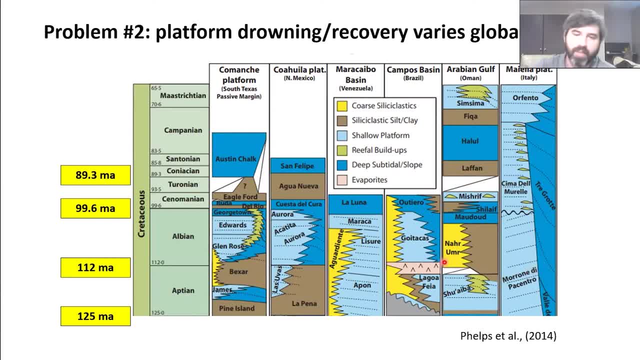 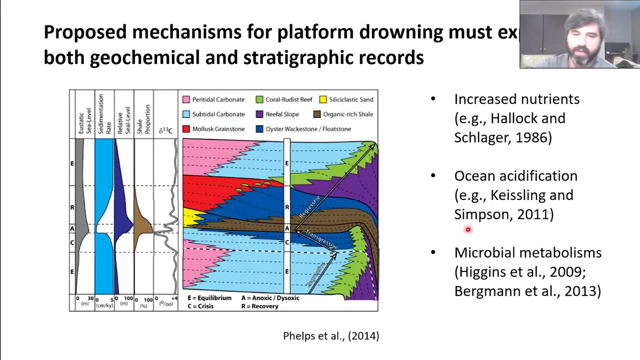 top. And so again, I just kind of it just kind of bothers me that that, you know, the ocean acidification story has this, this kind of really nice appeal to it. But I think there's room for at least one other mechanism, And so that's why I want to kind of highlight what we did in this work. 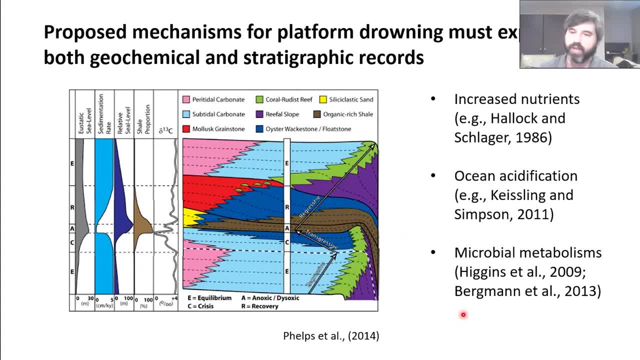 which is, we looked at another way at which you might generate drowning based on microbial metabolisms. And so, whereas the ocean acidification story kind of looks forward and takes elements from modern climate change and tries to project those into the past, this microbial metabolism story actually, 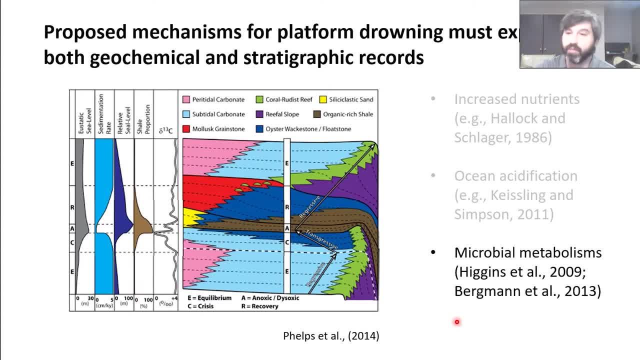 looks backwards And it looks back to that period of Earth history and the Precambrian, where there wasn't a lot of oxygen in Earth's atmospheres and oceans, and tries to maybe grab something of use out of that and then use it during these short term reversals in the Phanerozoic. 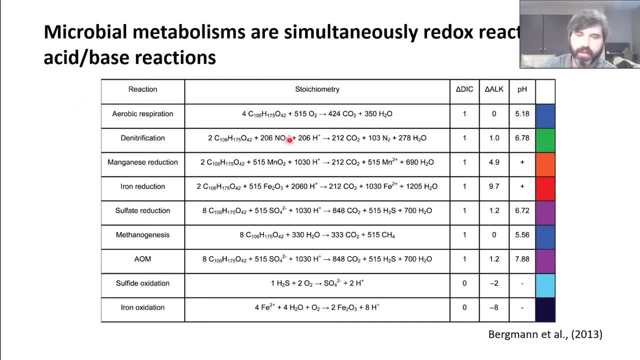 So I apologize for springing this on you early in the morning, But the way this usually works is: all these metabolisms are both acid-based reactions and redox reactions. That's important in terms of what we discussed earlier, because the redox reaction part of this. 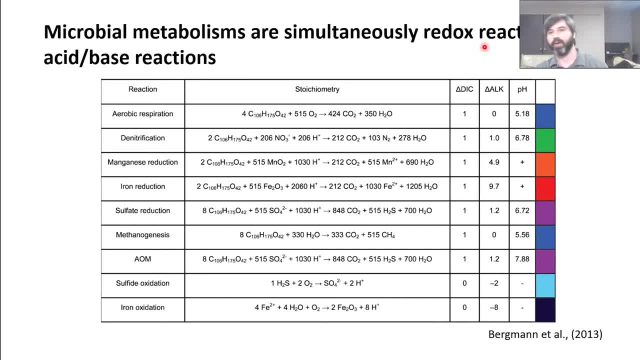 is what we know, or what we think we understand really well about the ocean's chemistry during these time periods, And so the kind of promise with this is that, hey, if these redox reactions are changing because of microbial metabolisms, that also implies an acid and base change. 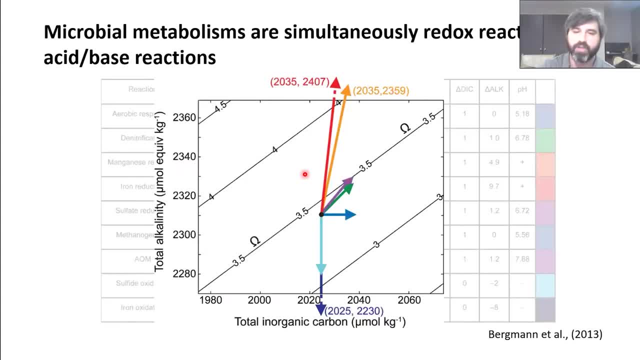 And so we're going to be able to do that. So I apologize for these, But the way this usually works is we take these kind of tables and then we plot them on a bivariate plot And then we represent each of these reactions as a vector. So the way these plots work is they have a horizontal axis. that 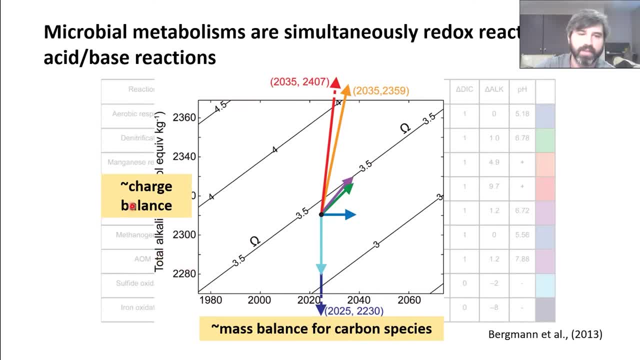 is a counting of mass balance for carbon species. They have a vertical axis that has something to do with charge balance, And then the vector shows the pathway for each one of these reactions and says, OK, if I respire a certain amount of organic carbon. 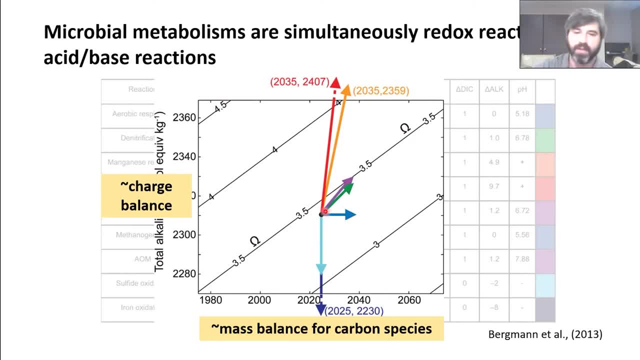 and convert it to an inorganic species like CO2, how much change do I get in the charge balance of seawater that accompanies that And what does that mean for the carbonate system? Again, I'm using this capital Greek letter, omega, which is a measure of how favorable or unfavorable carbonate precipitation reactions are. 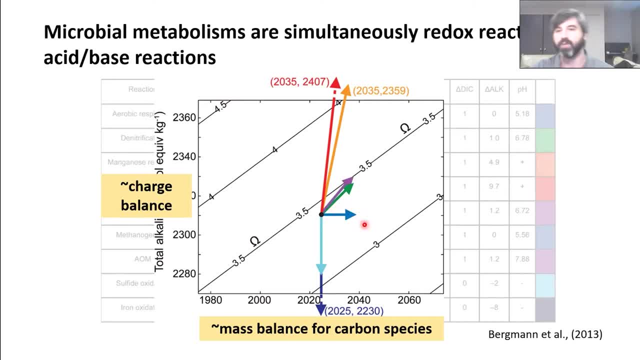 And the answer is: it actually really depends on which reaction pathway you're using, And the really important ones here are this dark blue arrow, which is aerobic respiration, And so, in the presence of oxygen, respiring organic matter makes a vector path. 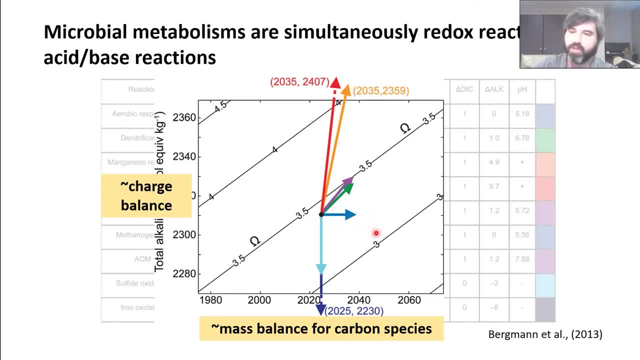 that pushes you toward lower contours of omega, And so usually you'll see these in studies of early diagenetic environments where organic matter is breaking down on the presence of oxygen, It tends to prevent carbonate cements from forming, And, in contrast to that, anaerobic processes or processes that use an 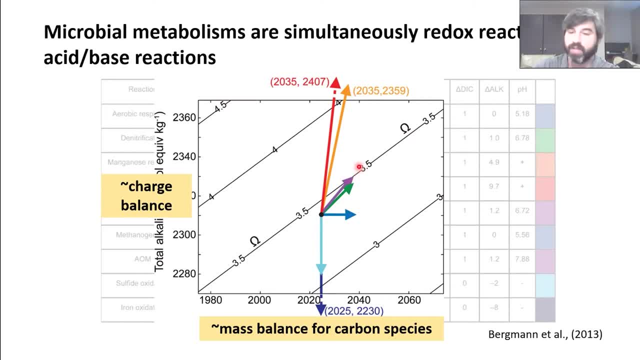 electron acceptor besides oxygen, tend to increase the saturation state, And so the one we'll be talking about in a moment is brass. It's Q8, the supreme form of copper ioniside, And, in contrast to that, anaerobic processes or processes that use an electron acceptor besides oxygen, tend to increase the saturation state. 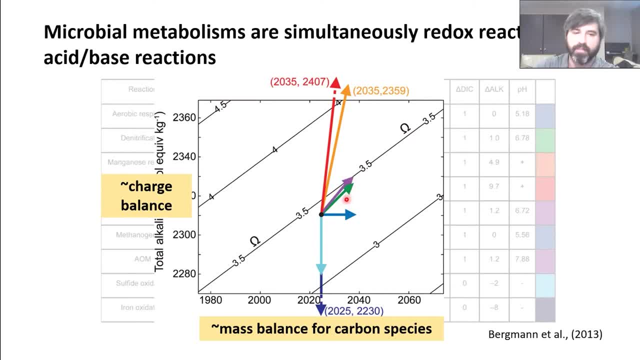 And so the one we'll be continually including here before me. This is quartz ion, is Auchi, betweenceğim and citric acid, which Значит that androgen- one we'll be talking about today- is um sulfate reduction, and so that's actually so. so the kind 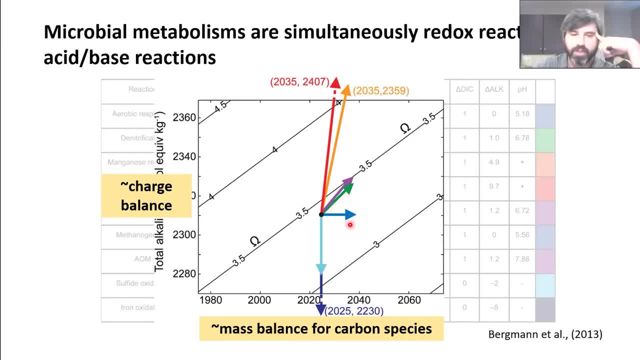 of idea here is that, well, if the oceans are changing their redox state during ocean anoxic events and that redox state correlates with changes in microbial metabolisms, that implies that the acid-base chemistry is changing in a way that we can reasonably guess at or model. 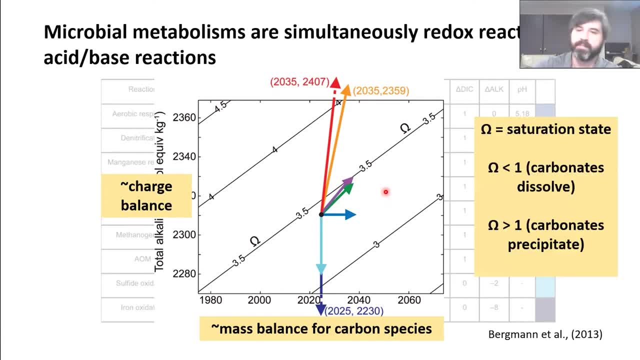 sorry, this is just a little side box about this. again, this capital, uh creek letter omega. it's the saturation state with respect to carbonate minerals. when that number is less than one, carbonate will dissolve, and when it's larger than one, carbonates precipitate. and then the you know. 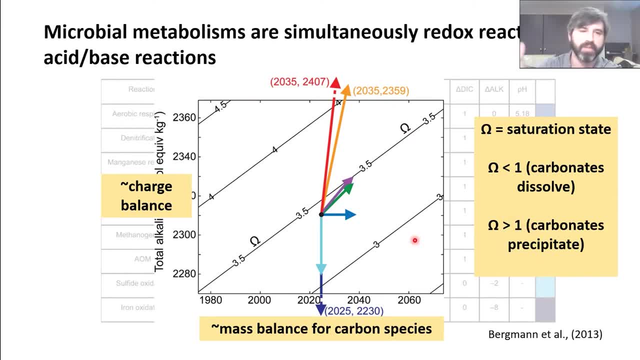 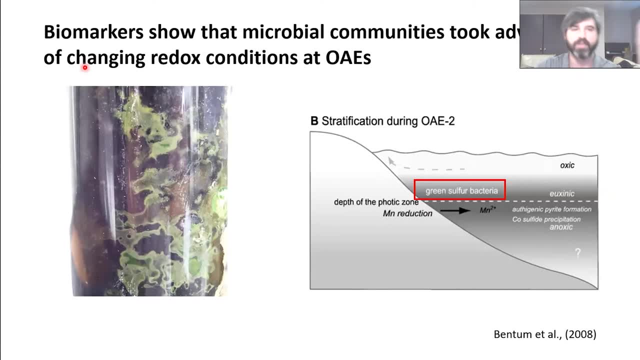 the value. the degree to which it's larger than one implies something about how fast or slow that reaction is. so just before we go on, you might ask the question: how fast or slow that reaction is? is there? is there independent evidence that these redox changes in the ocean are coupled to changes? 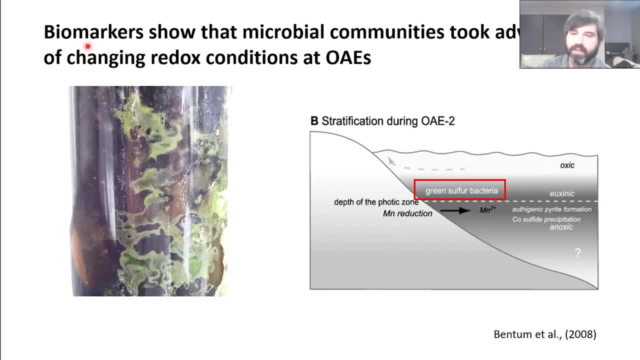 in microbial metabolisms and i would say yes. and the kind of data set that i turn to is a lot of these biomarker studies which are showing that these uh changes and trace elements that suggest redox changes are also coupled to changes in biomarkers that suggest different microbial 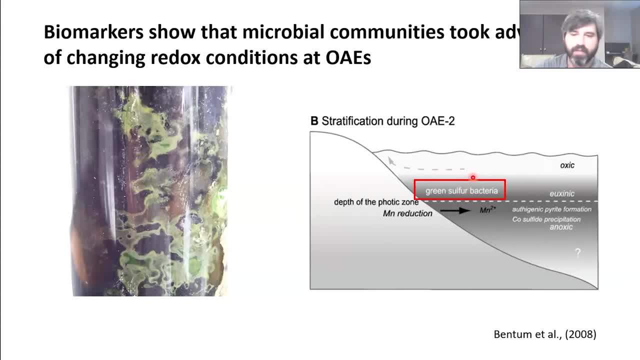 metabolisms, and the one that i've kind of seen come to light over the past 15 years or so, are these biomarkers, um derived from green sulfur bacteria, and so the way these green sulfur bacteria work is they need a source of sulfide, and then they need sunlight, because they're doing photosynthesis, just not. 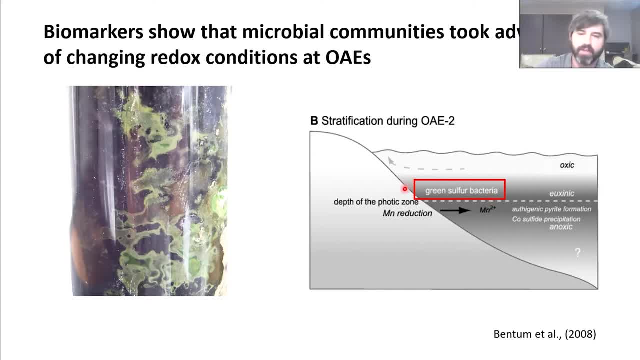 photosynthesis, like you learned in school, that produces oxygen, and so the kind of trick with these is: i need both light and hydrogen sulfide, and and that's those. two things would not be coincident. in most of the modern ocean, the typical place you find these is like in nasty hot spring. 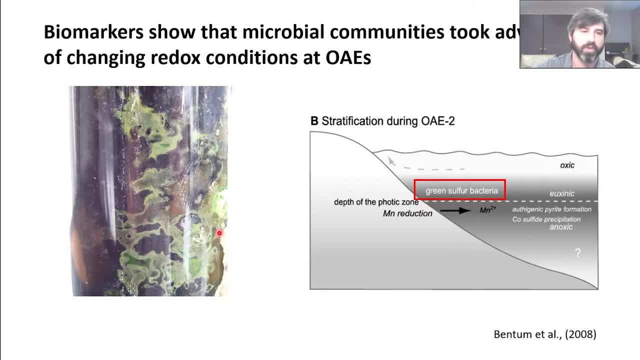 environments where water- anoxic water- is bubbling up from underground and then it's being exposed to sunlight very quickly. you don't expect to find it in the ocean, and yet for a lot of these ocean anoxic events like oae2, they're finding evidence of green sulfur bacteria in marine sediments, and so the typical interpretation. 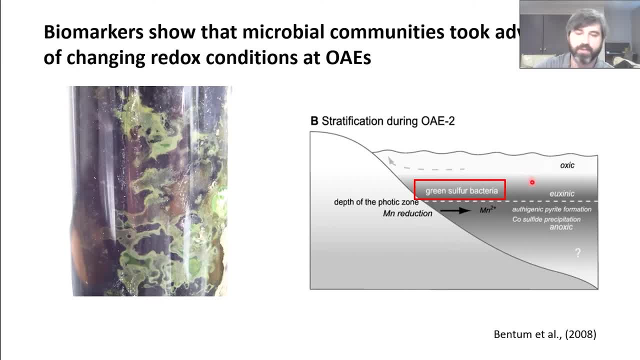 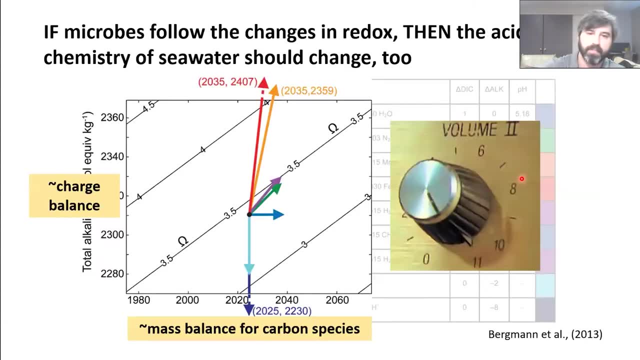 of that is that i have a very large pocket of sulfitic water and the top of that pocket is actually extending up into the photic zone. so again, i just want to come back to this idea of how we're going to treat this in this box model, which is: you know, we've got this, we've got these. 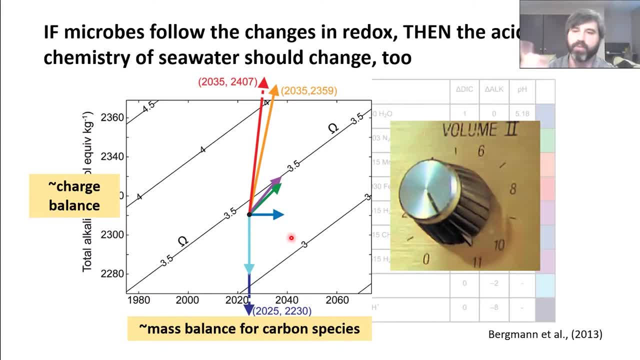 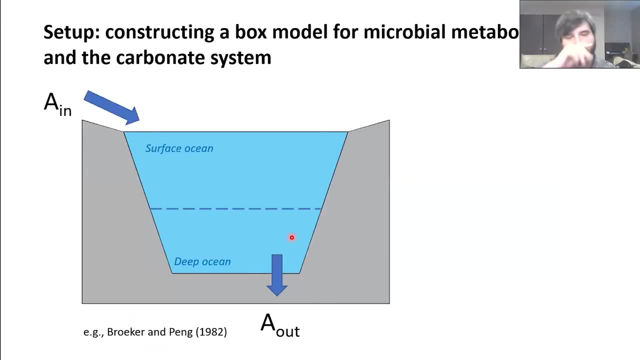 set of microbial metabolisms. they they are both redox reactions and acid-base reactions, and the idea is, if i'm turning that knob during an oae and i'm changing the redox, this implies that that also must change the acid and base chemistry. so let's move to the setup of this box model. 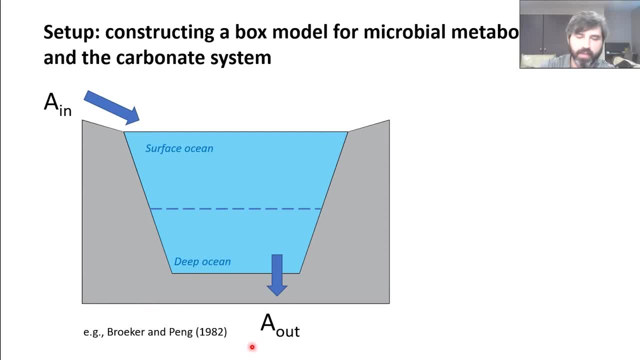 um, and so what i'm going to do is i'm going to use a. we're going to modify some pre-existing box models that are usually used for, like modern chemical oceanography research, and so the kind of first thing that these models have to do is they: they have to have a steady state, what i mean by that. 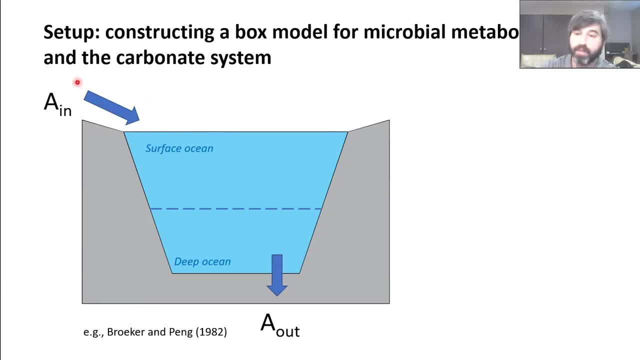 is that the inputs and outputs are balanced. so for an ocean model there's usually a weathering input, where material is coming into the ocean, dissolved materials coming to the ocean through rivers and runoff, and then every year there's a budget of weathering and then the same amount of material. 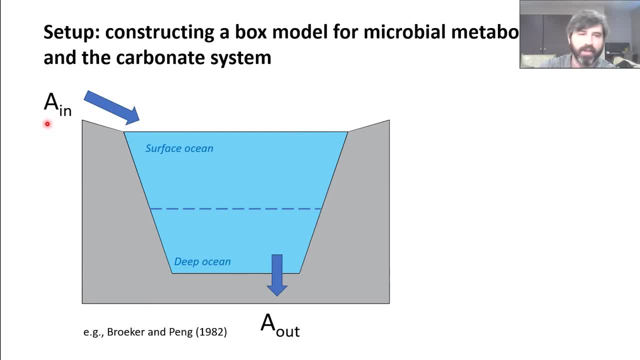 leaves the ocean. so for something like carbon, you know, uh, inorganic carbon species might make their way into the ocean, and then, every year, the earth's carbonate budget and its organic matter budget need to be balanced so that we don't have a runaway system where the um, you know. 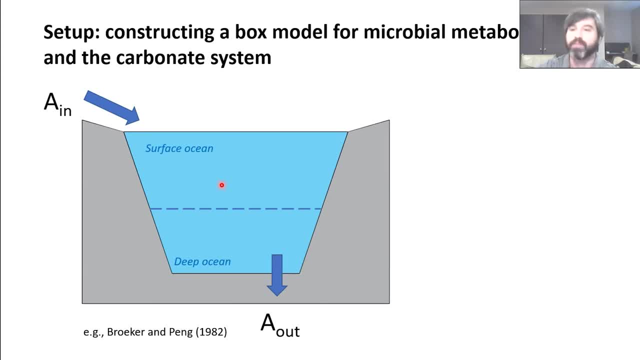 concentrations within this box increase or decrease forever, you know. so usually the starting assumption is one of steady state. um, here i've labeled the weathering: uh a in for alkalinity. um, usually we start by balancing uh kind of the weak bases that are being brought in to sea water through. 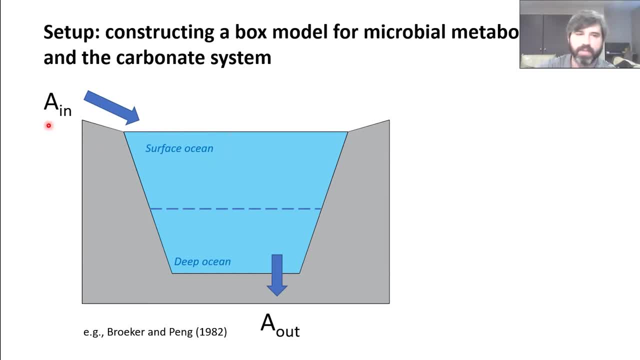 weathering, and so this is typically the way this is written, which is like a n equals a out. these outputs need to be balanced. however, there's this kind of like wrinkle in there that there's internal fluxes. if i have more than one box in this box model, there can be movement between. 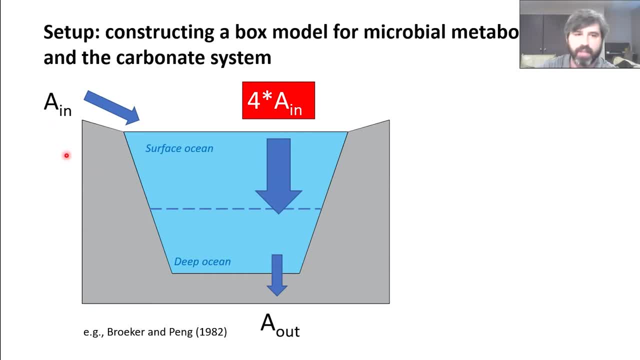 those boxes that that you know don't necessarily upset the balance between inputs and outputs. and- and If you talk to a chemical oceanographer they'll tell you that you know, if I have this weathering budget of alkalinity, about four times as much alkalinity leaves the surface ocean as comes in every year. 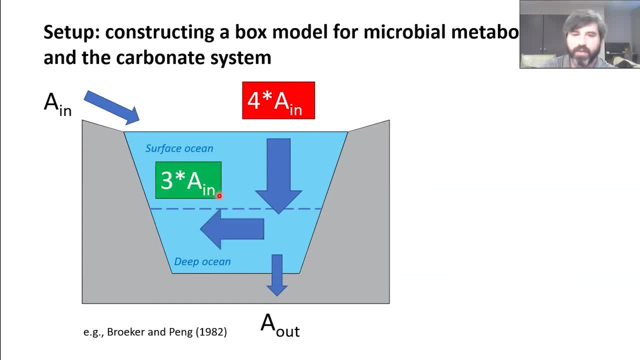 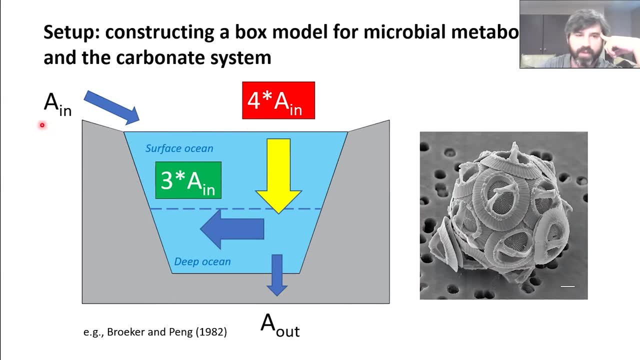 And a lot of that leaves either as carbonate platforms or as these kind of little coca leaf chocks And so so the kind of the way this works is okay. if I'm, if I have four times as much alkalinity leaving as comes in, I need to somehow return most of that to the ocean before it reaches the rock record. 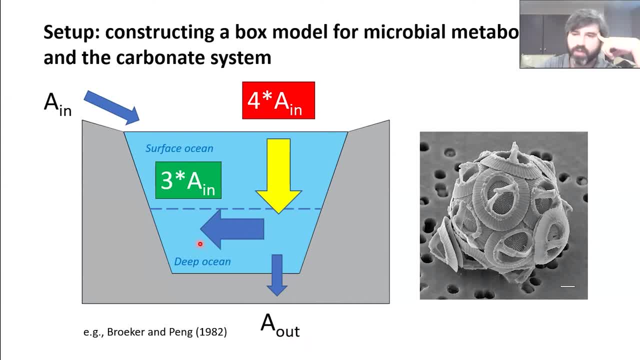 And that's, that's actually what happens, which is, the deep ocean actually dissolves carbonate quite efficiently And so of this four times flux that that leaves the surface ocean about three times, three times the weathering input Is redissolved. 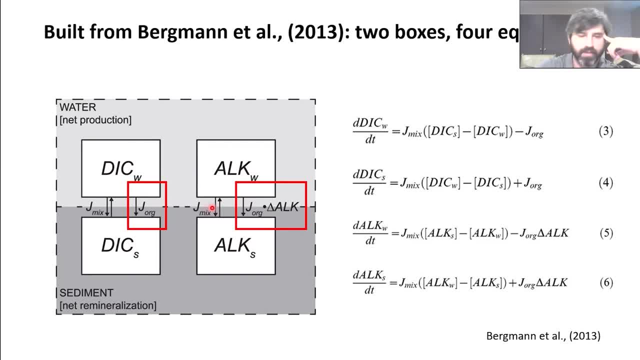 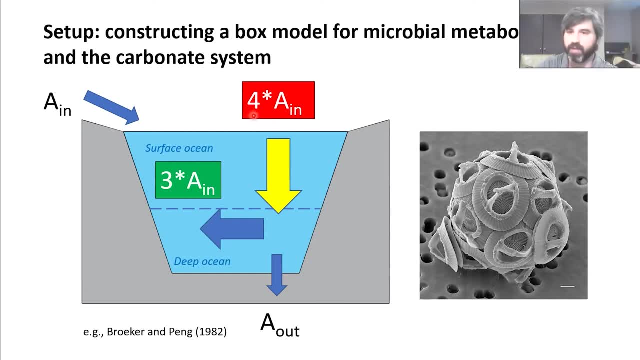 Okay. So what we did is we decided we wanted to. sorry, let me. let me go back for a second. So this, this answer is non-unique. I started with four because that's what the modern system suggests, but there are other combinations that would give you the same A in equals A out. 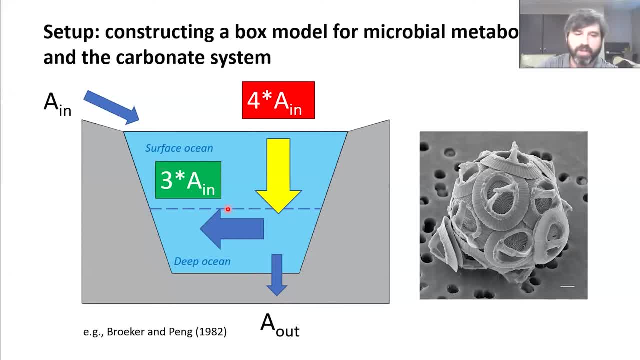 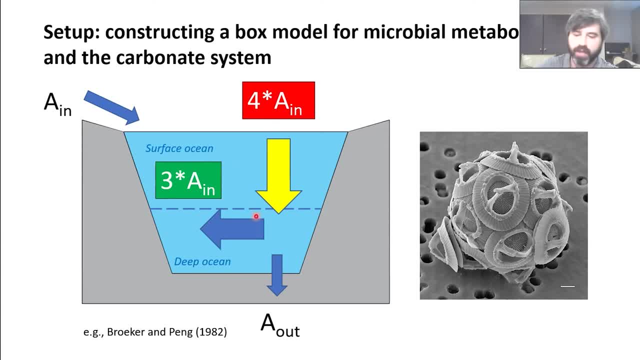 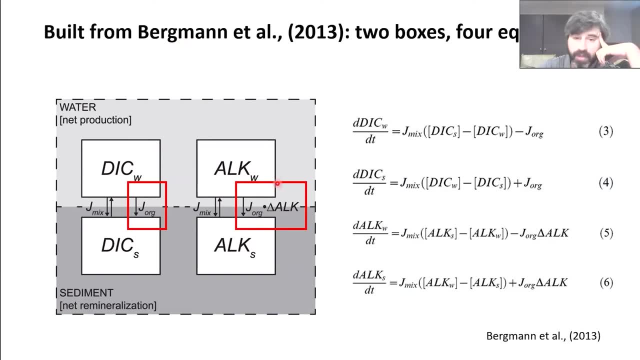 You know, make a new balance between the two, the two boxes. So what we did is we worked from a preexisting box model. This is from Kristen Bergman's work at MIT And she had kind of come up with a box model, that again drawing from the past. 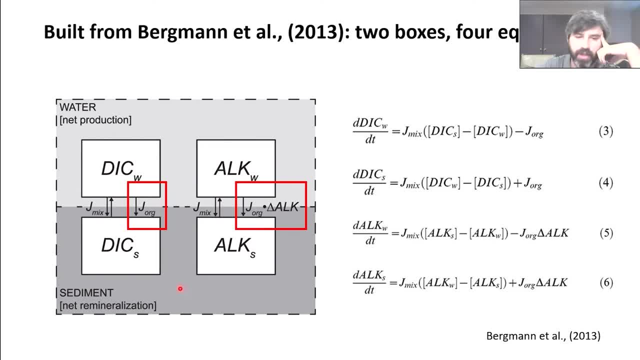 Her work is really focused on the protozoic and trying to understand how microbial metabolisms would work across two boxes, In this case the sediment water interface. So I don't, you know, really think it's helpful to go over the. 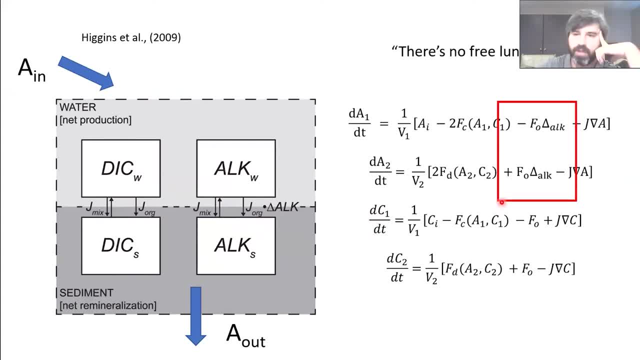 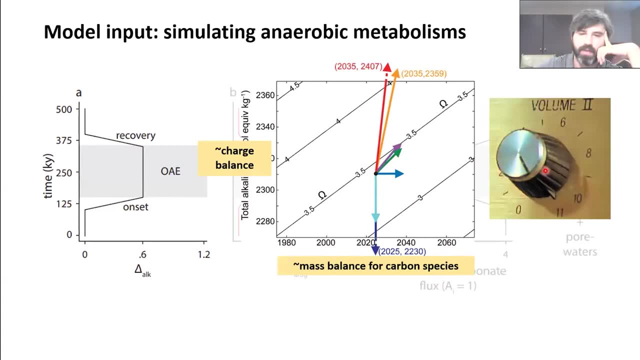 Equations too much, except that I'll point out that the term that we'll be talking about here, which is this capital, Greek Delta- And in our model that's the knob that we're turning, that represents the microbial metabolisms. So the way we're going to set this up is we're going to, we're going to let this model run at steady state. 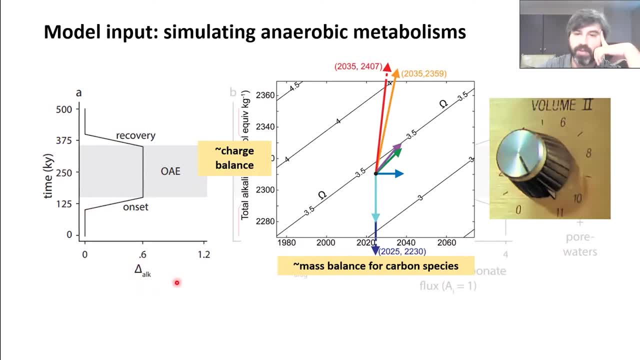 And the starting value of this capital. Greek Delta represents an ocean that's full of oxygen, where almost all organic matter is being respired with oxygen as a primary electrolyte And again that implies a certain pathway and a certain ratio between mass and charge balance contributed when I respire that organic matter. 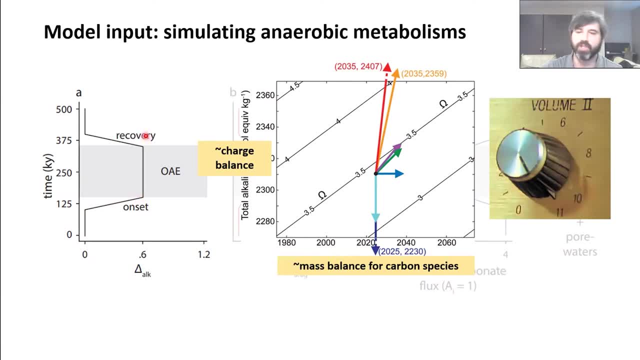 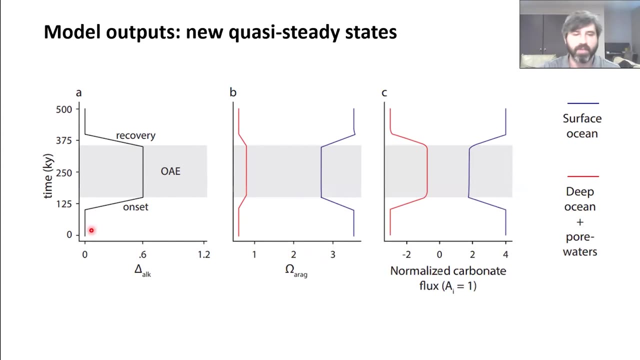 And then what I'm going to do is I'm going to simulate an ocean anoxic event by turning that knob and representing a mixture of oxygen and another process like sulfate reduction. And so what we found is, you know, when we, when we set up this box model, changing the 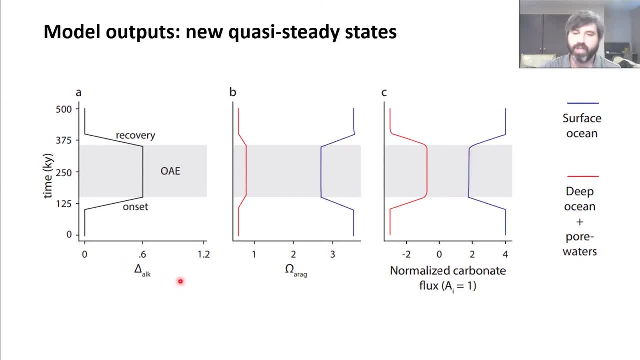 Without, without changing anything else, changing the, the way that we're representing microbial metabolisms that actually changed the way that carbonates were precipitated and dissolve between the two boxes. So here I have this capital Greek letter, Omega, And there's two curves here. the blue curve is for the surface ocean, so that's that top box in the model, and the red curve is for the deep ocean. 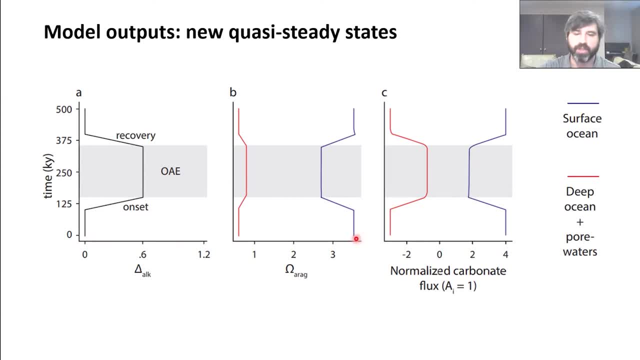 And so in the in the starting state. in a world with without oxygen, the distance between The saturation state and the surface ocean and the deep ocean is very large. There's a very high saturation state in the surface ocean that's balanced by a very low saturation state. 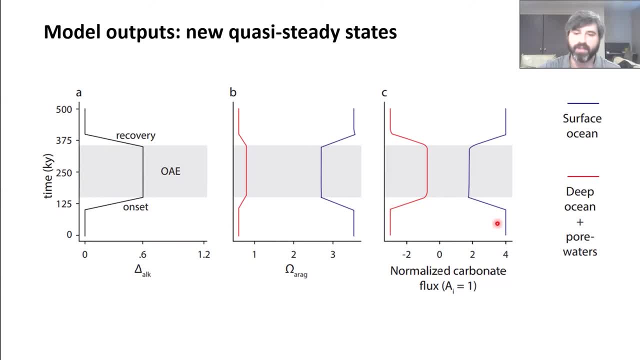 And if we kind of cast that in terms of fluxes, that's the situation where I'm producing four times as much carbonate as I need to produce in the surface ocean and I'm dissolving three times as much During the ocean anoxic event. 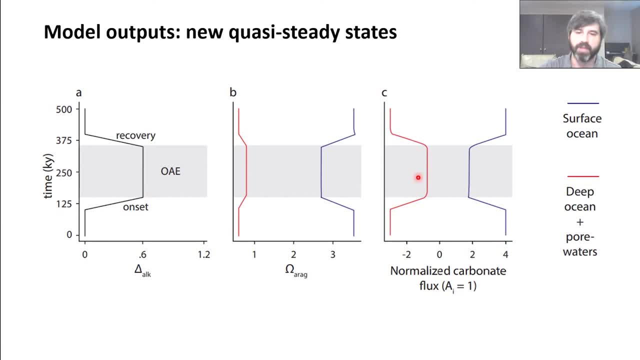 These, the contributions of these anaerobic microbial processes, Actually reduce the dissolution of the deep ocean, and what happens is that the Kind of fluxes in the surface ocean eventually reduced to match that, And so the sum of the sum of these two curves- actually the difference between these two curves- is always one. 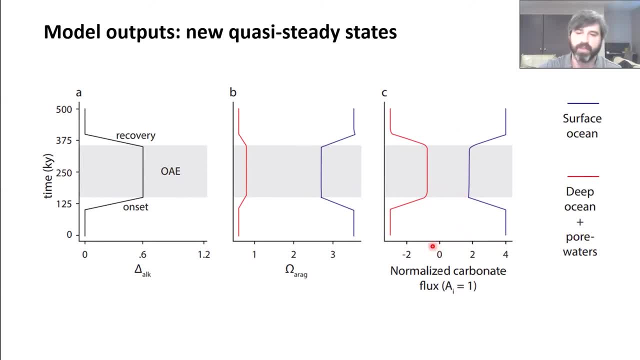 So this is normalized, that weathering input flux, and so this is kind of that expression of multiple valid steady states. And the most important part of this, The most important part Of this model, is the fact that, you know, I have kind of assigned an arbitrary timescale to this OEE. 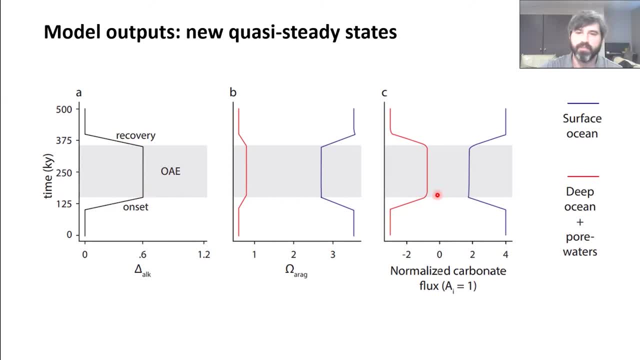 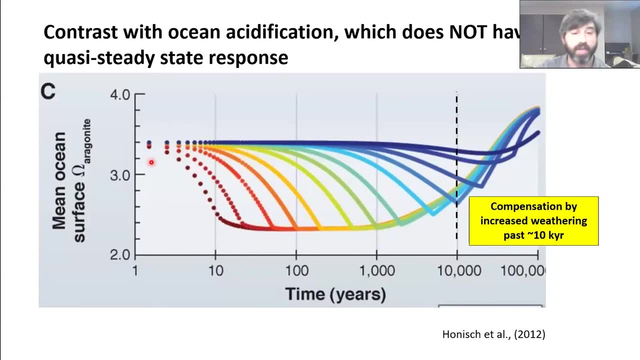 But you'll notice that the the shape of the input curve pretty much exactly matches the shape of the output curve. And what I want to do is I want to contrast that to the ocean acidification model, because what we saw there is, if I disturb the system, there are very, very strong negative feedbacks that start to push the system back to its starting state. 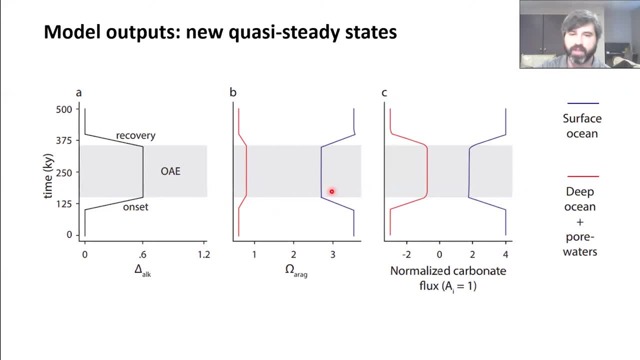 And the kind of drowning mechanism We're proposing- proposing here- doesn't do that, and in fact, the ocean only return to a starting state once I flip that knob back to a starting condition. So what this means is that this operates over arbitrarily long time scales. if I had chosen to make this OEE a million years, 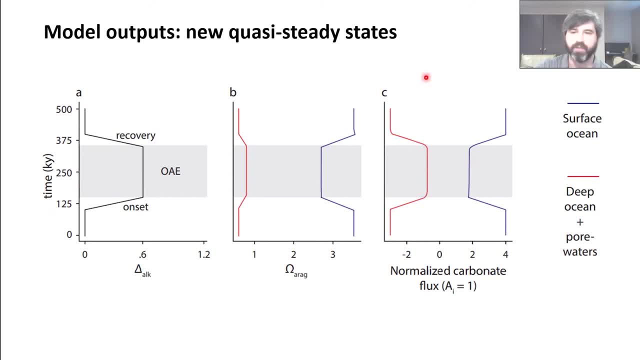 Then this carbonate, these carbonate fluxes, would have persisted for a million years. and what it does is it effectively couples this very short term carbon cycle at Earth's surface to Earth's very long term redox cycle, which tends to operate at these longer timescales. 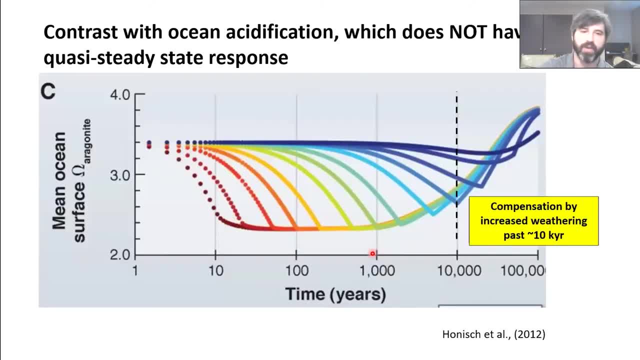 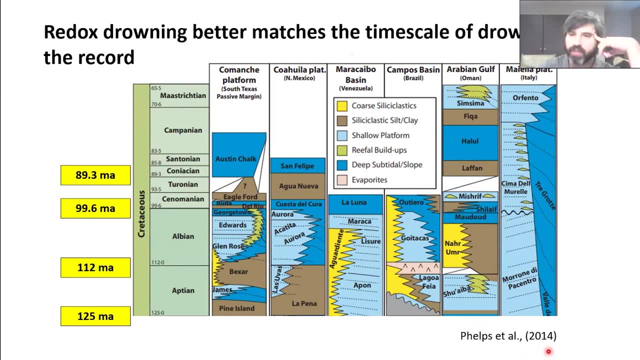 that kind of match what we see in the stratigraphic record. And again, I just like this is- I just want to point out this is: this is all motivated by stratigraphy, you know it's is motivated by the stratigraphic record of these events. and so, to me at least, this checks at least one box, which is that 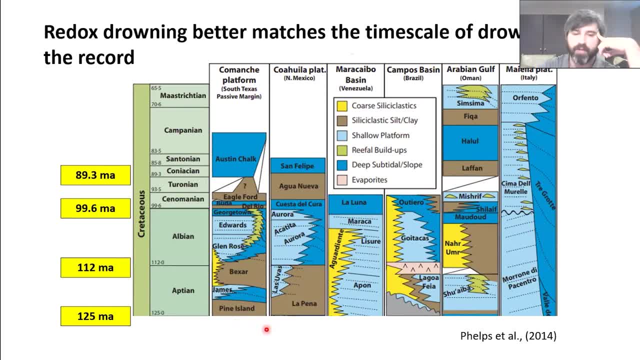 This process is capable of operating over the long time skills that we see for the drowning events in the stratigraphic record. What I didn't cover today, and what isn't really covered in this model, is that you know, although we chose to represent the entire ocean as two boxes, we could have subdivided that. 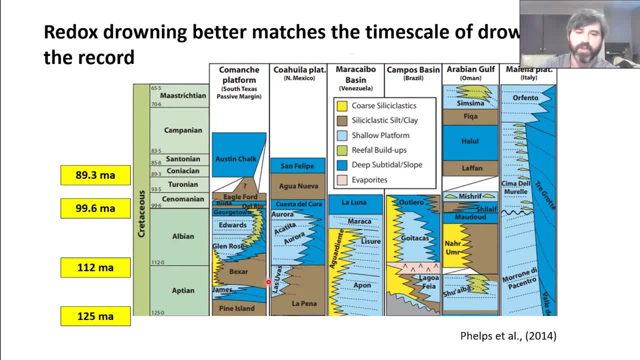 further, and so that kind of gets at this secondary issue of: well, you know, a lot of these drowning events are not synchronous, and so you know that I kind of picked on that. for the ocean acidification model, I would say that our proposed process might actually be able to generate this if we were to. 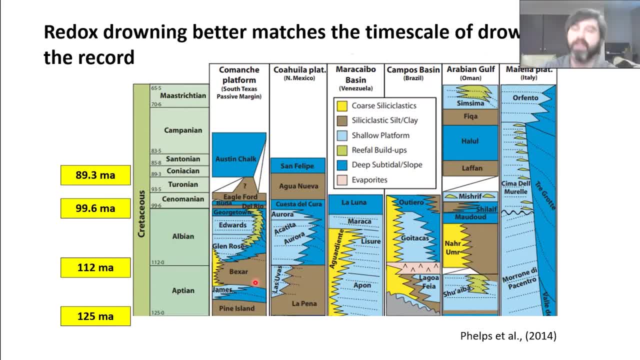 subdivide that model into boxes for different ocean basins, and so I think there's a kind of promise that you know this. this might actually better match the heterogeneity and time scales of the stratigraphic record. Okay, so kind of the last thing we did is we wanted to generate 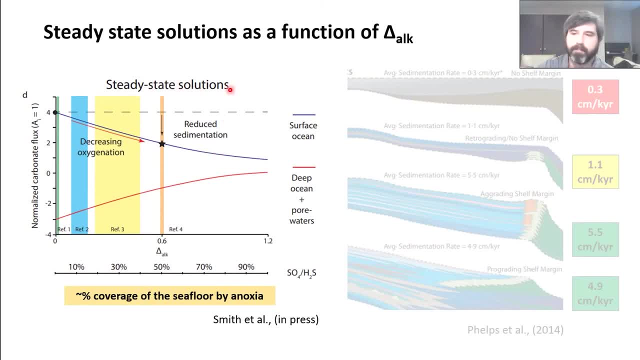 a series of steady state solutions. so you know, we said that the time variant solution tends to go towards a new steady state, and so you know, what I wanted to do here is really distill everything into a curve or a set of curves that I could use to explain platform drowning. 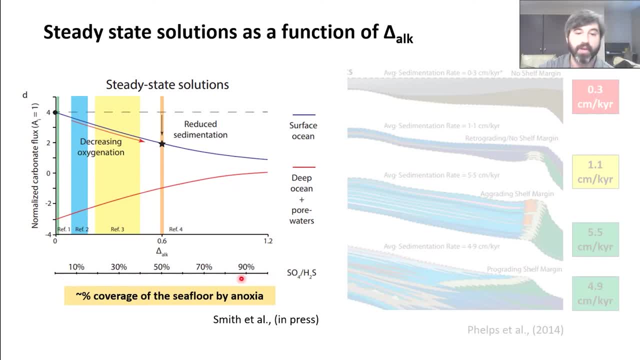 And so what we have here is we have a new horizontal axis, which is the amount of oxygen that's been replaced by sulfate as a primary electronic sector, and here I'm going to make the argument that that's roughly analogous to the percent of the seafloor that's covered by 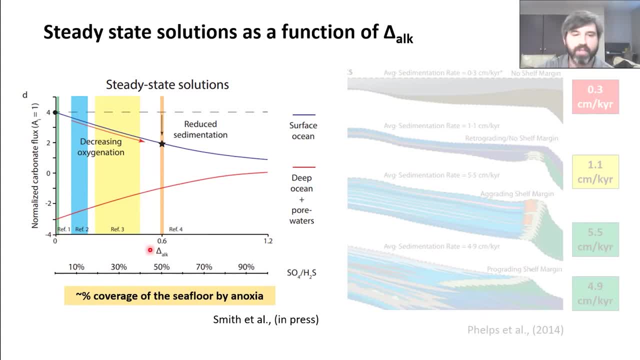 these anoxic water masses, and that's actually something I wouldn't say it's known from the stratigraphic record, but those are things that people have estimated using different trace element systems, isotope systems and biomarkers. And so what I did is I kind of dug through the literature and I found estimates going from about 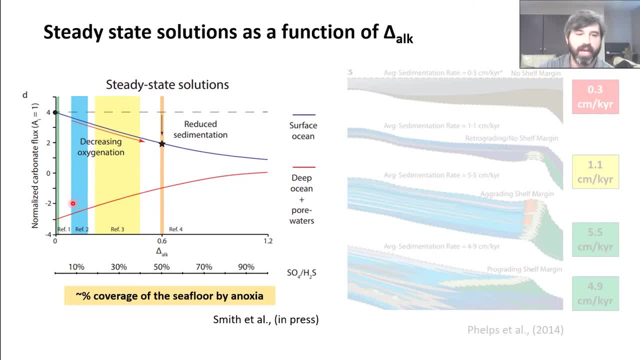 eight percent, you know, or a couple percent to maybe ten percent of, uh, you know, the seafloor covered by anoxic water masses and then if you use the biomarker data, that suggests maybe even fifty percent of the ocean's floor during ocean anoxic event two was covered by these anoxic water. 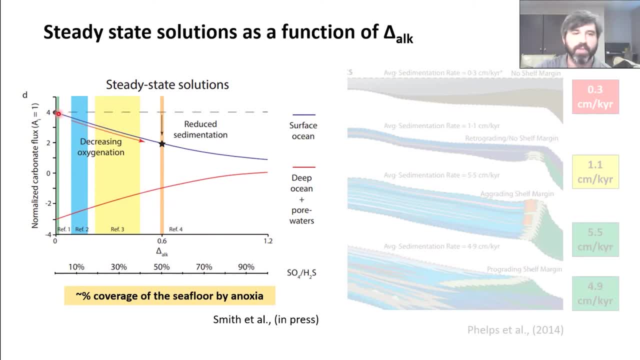 masses. What I've done here is I've plotted the kind of difference between the surface ocean and the deep ocean as a function of how much of the ocean's floor is covered by the anoxic water masses. So I would say that the left, uh the leftmost side here is is a representation of what our earth looks like today, where virtually all of the ocean's floor is covered by oxygen. and then the right here would be the latest pre-cambrian, where we think there's, you know, still very little oxygen in earth's oceans and that most organic matter is being respired by. 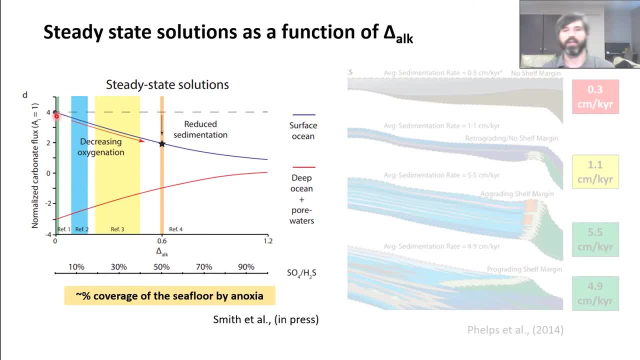 sulfate reduction, And so again, I kind of mentioned the beginning of the talk. I don't think it's possible to go all the way back to the pre-cambrian during these short-term reversals, but you start to get there and what this plot does is it kind of quantifies how far along. 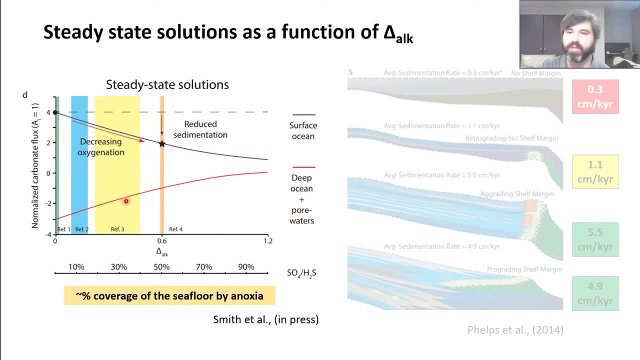 that process you are and what that means for the surface ocean and the deep ocean. And so this blue curve here is, the is the surface ocean, and so it starts at a four times overproduction of carbonate, which is again based on kind of modern chemical oceanography. and as I start to increase the, the 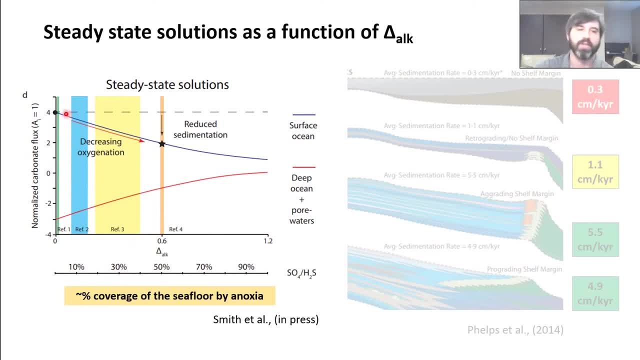 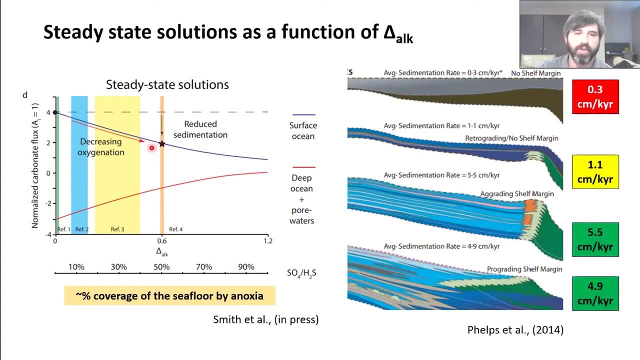 coverage of the ocean. I'm going to start to see that the surface ocean is going to be more and more sedimented, And so what I would do is I would look at this and I would say that's a valid explanation for platform drowning. You know, if I'm trying to kill these platforms by taking away 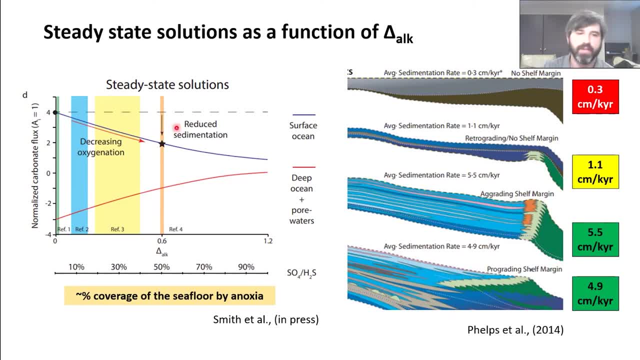 their ability to keep up with the background subsidence rate, then this is a valid mechanism for that, And I want to point out one last thing, which is that the shape of these curves is slightly concave up, And so if I'm trying to kill these platforms by taking away their ability to keep up, 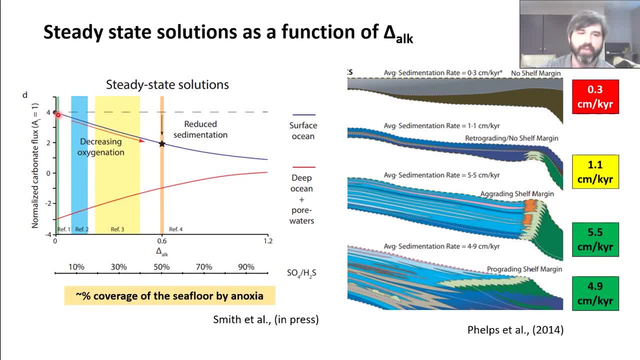 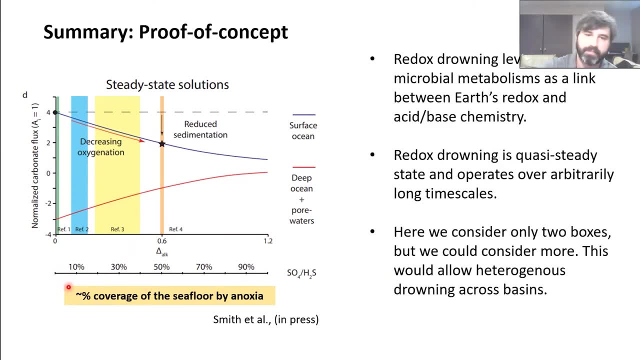 and what that means to me is that you actually get the greatest rate of change, You get the most damage to the carbonate system during the early spread of anoxia. So just kind of a summary. you know, this study is really kind of a proof of concept. You know, just kind of tugging using a 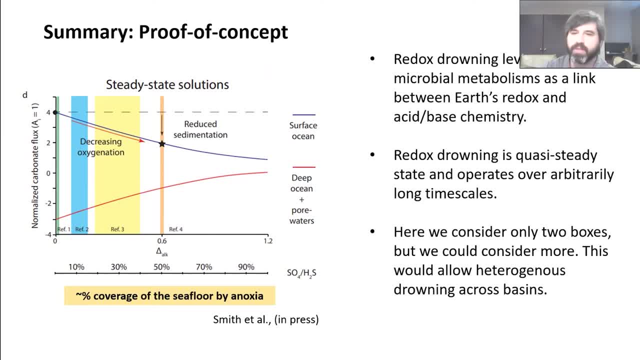 box model to tug at the strings that connect different parts of the earth's, the earth system, and then, just like a gut check of whether this is, you know, thumbs up, thumbs down, looks like some of things we've seen, And so I'm going to start to look at this, and I'm going to start to look at 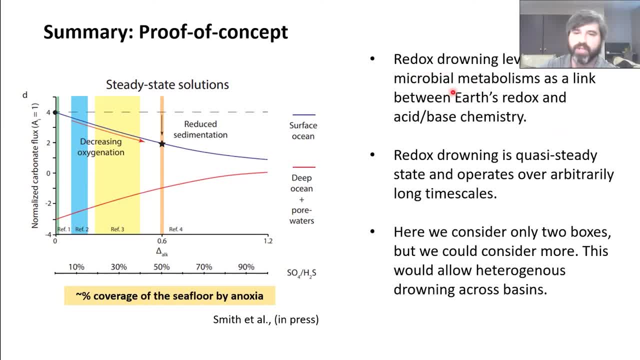 what we've seen in the stratigraphic record. So again, redox drowning leverages this kind of intrinsic link between earth's acid-based system and its redox system, which is provided by microbial metabolism. The mechanism that we're talking about is quasi-steady state and it operates over 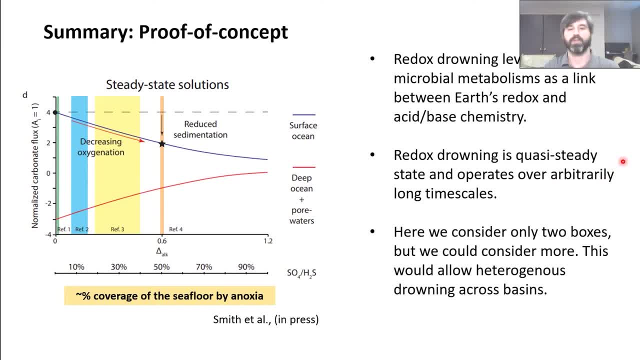 arbitrarily long time scales, which is good because it helps us match those kind of hundred, thousand year and million year time scales of stratigraphic record. And then this last part is not really something we did in this study, although we suggested it at the kind of at the end of our 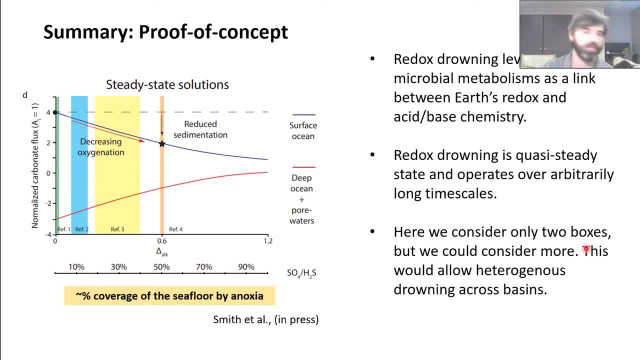 paper, which is, you know, here we're really considering only two boxes, which is this well mixed surface ocean and this well mixed deep ocean. But if I was to subdivide that into different ocean basins- for like the tethys versus, you know, you know, different kind of sub basins- I might be able 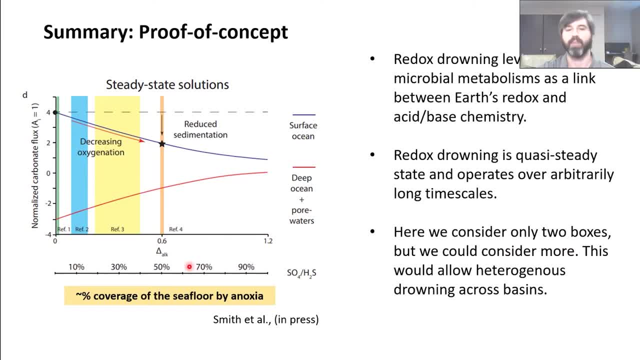 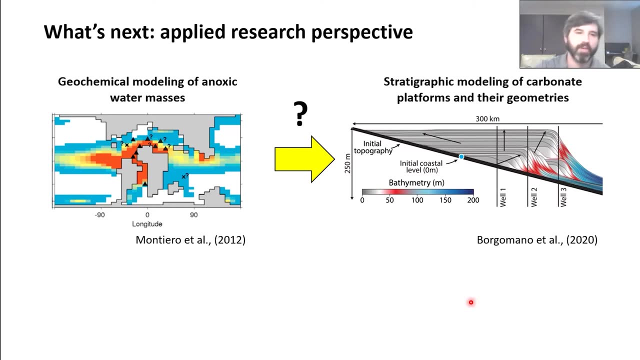 to sustain different curves in those different basins And that might kind of act to produce this differential drowning record that that is different, you know, both between basins and maybe within this the same basin. Okay, so with that I just want to take a little bit of time to talk about you know what's next. 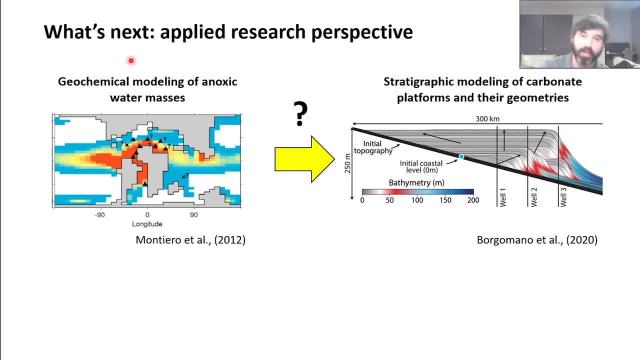 Like what? what are the kind of takeaways from this, from both the applied petroleum systems perspective and then from the earth history perspective? So I kind of started this talk in my background during my PhD. It was mostly in the kind of large-scale stratigraphic. 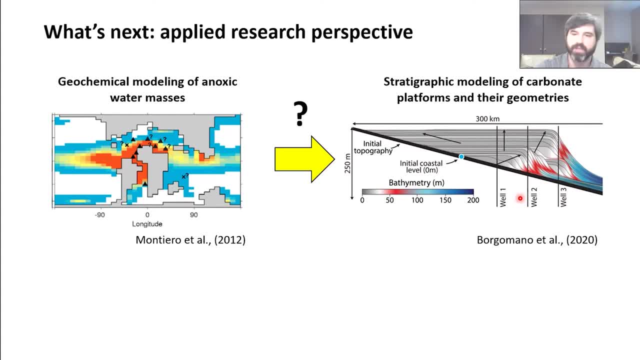 architecture of these carbonate platforms, And that was the motivation for this And the project. I would say we didn't really get all the way there, But the way that I would pitch this is: you know, there's different kinds of models. One kind of modeling, that's done. 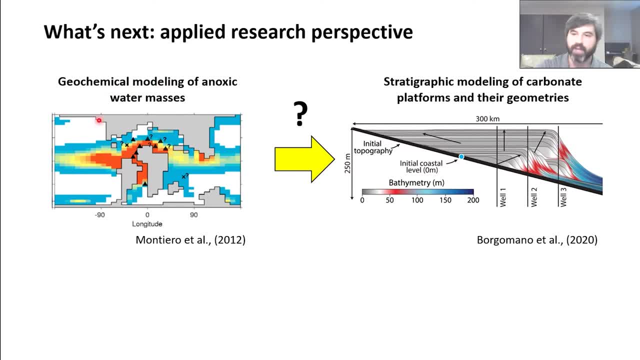 for these, these events, is this geochemical modeling of anoxic water masses. This is from a what's called an intermediate complexity earth model And they're they're trying to. the warm areas here are where they think there was anoxic water masses during OAE2.. And then on the right, 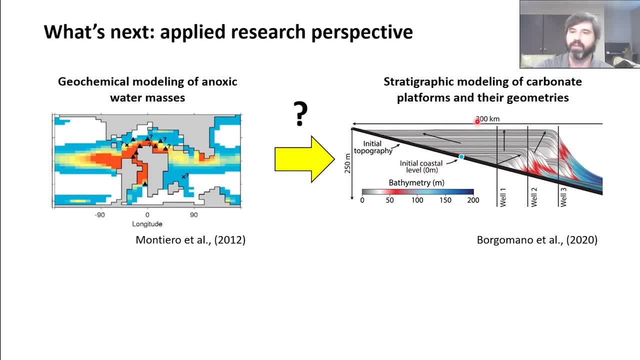 here I have a totally different kind of model, which is a stratigraphic forward model, where people, you know, they impose a sedimentation rate, They impose different subsidence rates and sea level, change history And they try to match the architecture of stratigraphic packages. you know, based on these models And and it's always a challenge to do- 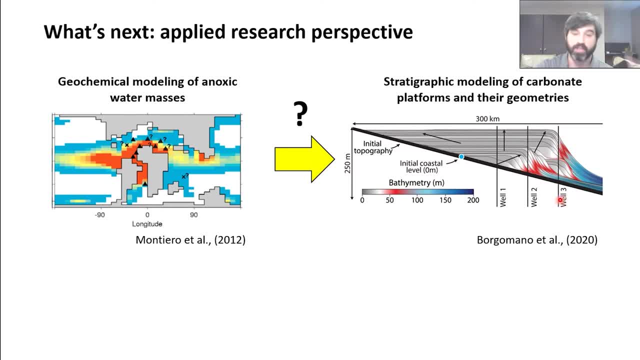 these in carbonates because you know it's easy to impose a tectonics history or sea level change history. But the idea of changing the carbonate sedimentation rate and how that responds quantitatively to the to changes, chemical changes in the ocean, I think is not well understood. 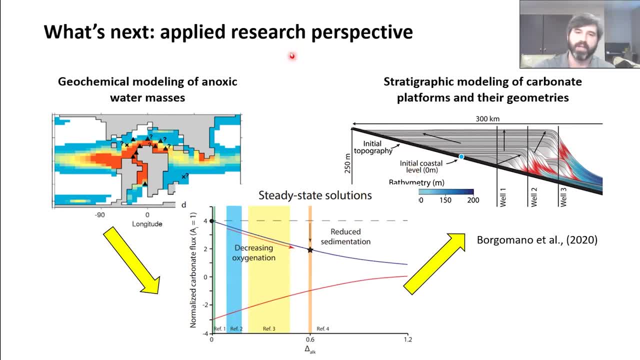 And so what I would do is, you know, I would propose this study as an intermediary that kind of sits in between these two approaches. It doesn't really get all the way to stratigraphic architecture, But what you can imagine doing is saying, okay, I'm going to take the output of one study, which is the amount of seafloor, that's. 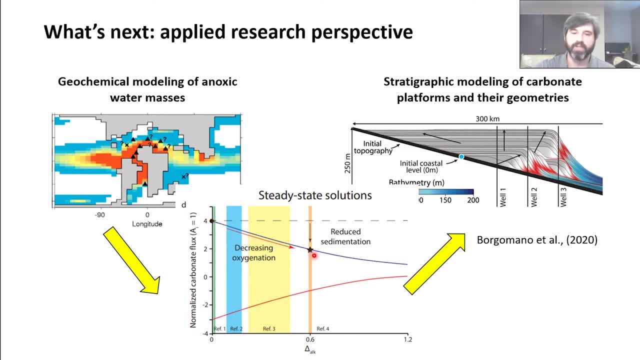 covered by anoxic water masses. I'm going to trace where that sits on this plot And then I'm going to come into this stratigraphic modeling program And I'm going to simulate an OAE by reducing the carbonate sedimentation rate by a specific amount. So for OAE2, I would like to 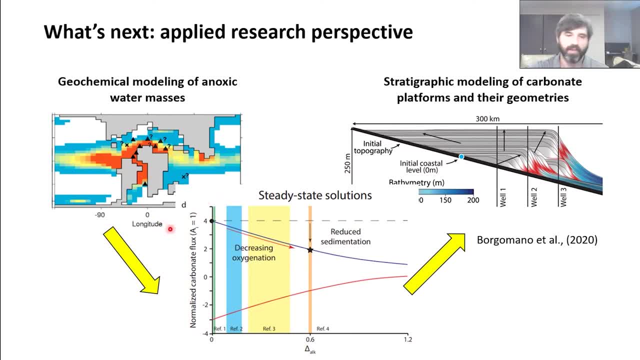 look at this study for OAE2.. I would say you know I've covered up the name here, But Monteiro et al suggested that at the peak of OAE2, 50% of the ocean floor was covered by sulfitic water masses. 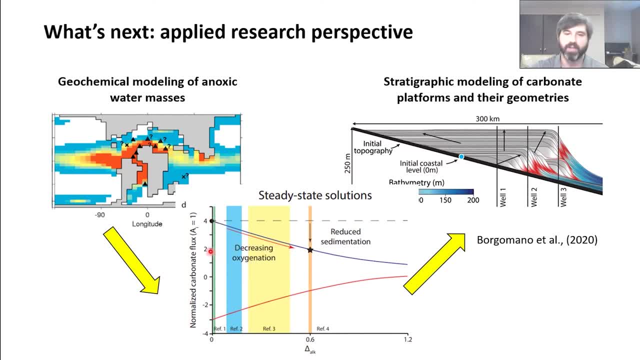 I come here on this plot and I say that's about a 50% reduction in the carbonate sedimentation rate in the surface ocean. And then I would come into my stratigraphic modeling program and say: you know what happens to the stratigraphic architecture of these platforms if I, halfway through this run cut. 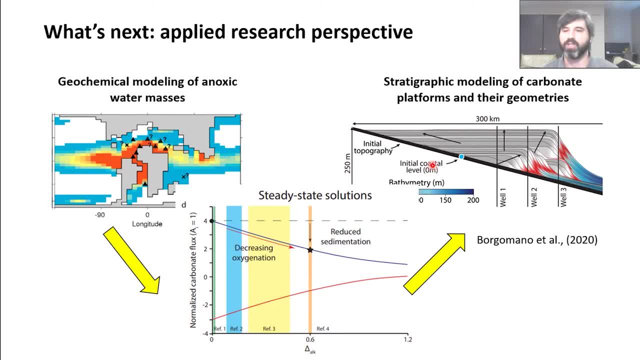 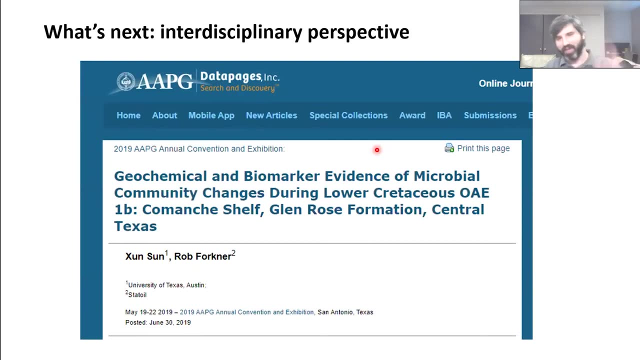 the sedimentation rate by 50%. You know what kind of patterns and geometries and scales are associated with that. And then you know, is that starting to get at what I see in the stratigraphic record and kind of the seismic scale architecture of these platforms. Another really, really interesting takeaway that I got from this: 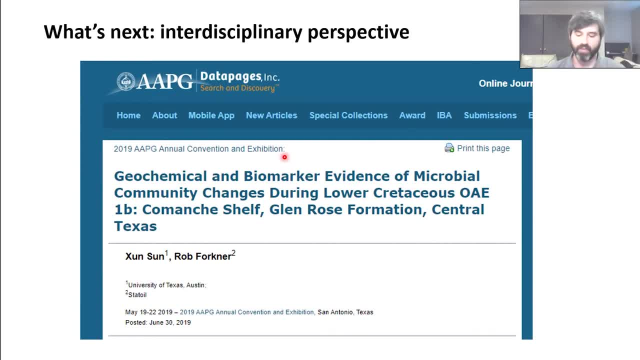 is again, you know this is leveraging the kind of redox history and the part of the OAEs we think we know really well. And you know, again, my background is mostly in carbonates but I found myself, you know, looking at biomarkers, I found myself thinking about organic matter and I think this is a really interesting 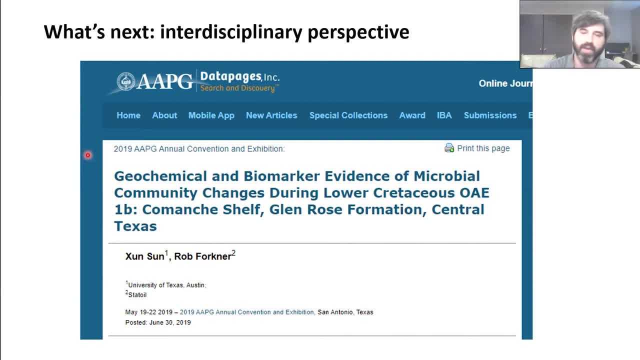 thing for the Bureau of Economic Geology, because you have all these like these interconnected research groups and there's, you know, people here like Bob who's made an entire career of understanding both carbonates and mud rocks. But I found myself wanting to leverage material from the kind of mud rock and unconventional literature to help me understand. 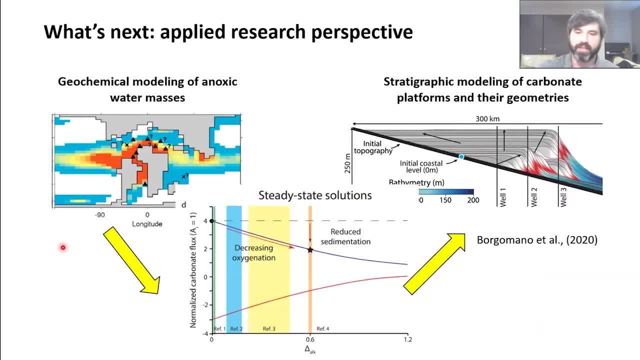 carbonates. And so you know, when we come back to this idea of: okay, if I have a stratigraphic package that I think is related to an OAE, how am I going to tell that, apart from a drowning, that's related to tectonics? 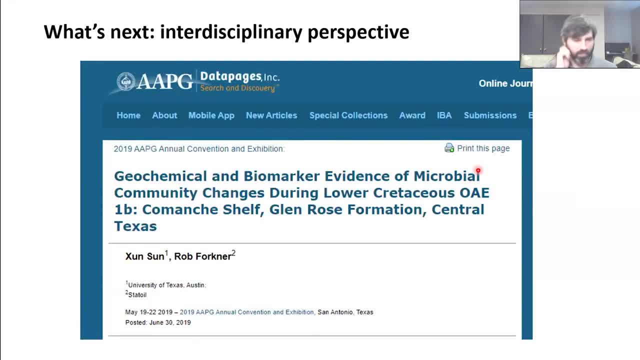 or to sea level, And I would say: well, show me what the biomarkers are doing in the basin, because this particular model that we're proposing is very much connected to microbial metabolisms and what you know. the first thing I'd want to see if someone was to apply this model would be: 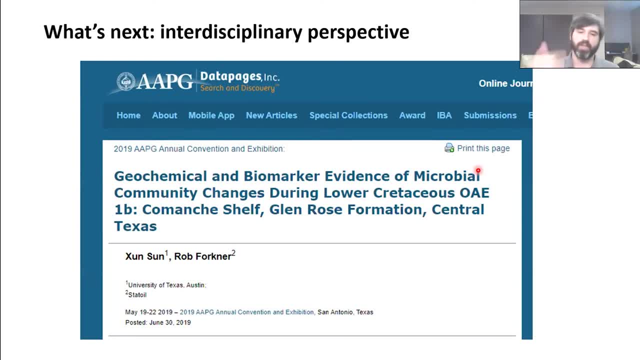 show me biomarkers that are saying not only is the redox changing, that the microbial communities are along for the ride and they're also changing. And I think it's really interesting that the Bureau has the relevant expertise both in carbonate systems and in kind of mud, rocks and biomarkers, to kind of make these studies work. 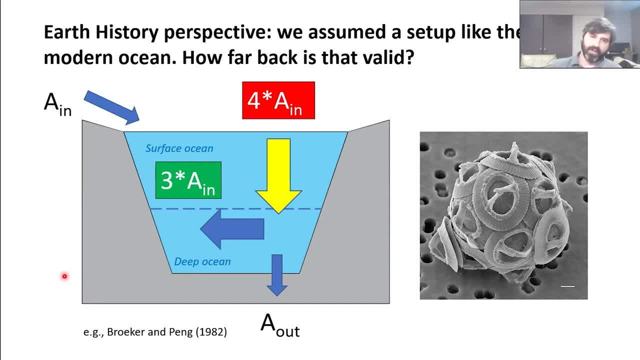 Okay, and so the last kind of element here is: again, I want to, I want to return to this earth history aspect, because that's that's my research, that's what I'm passionate about, And so, you know, one of the things you always have to do with these models is you have to ask what assumptions you 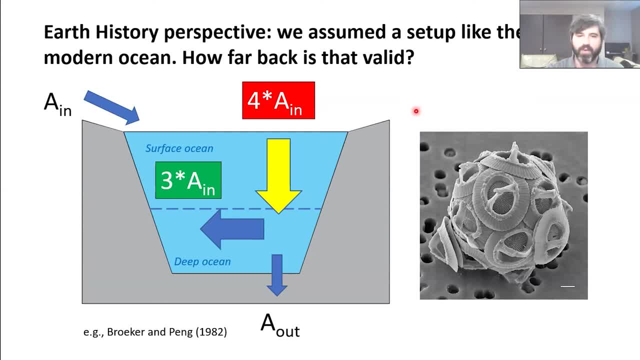 made and you have to ask, you know, when are those assumptions going to be valid and when are they going to be violated or invalid? And so one of the things that was- was we really leaned on for this- was again this: this idea that the modern ocean has this four times over production of carbonate. 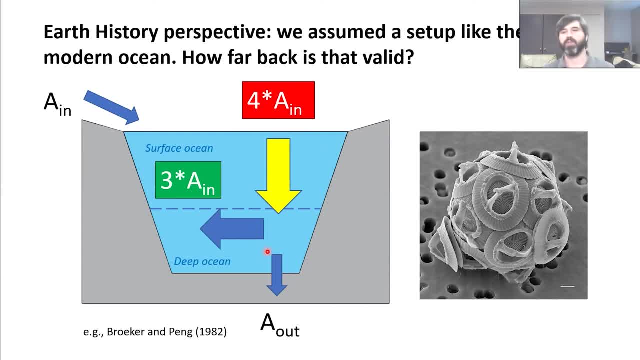 and that a large amount of that carbonate gets exported to the deep ocean where it can be resolved. And the way I've interpreted this is that a large part of that flux is in coccolith shocks. You know, it's, it's. it's not all in. 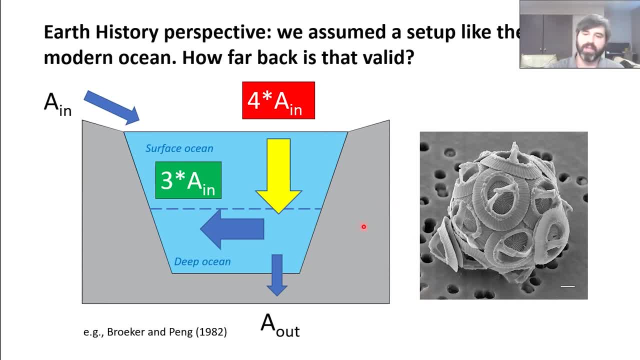 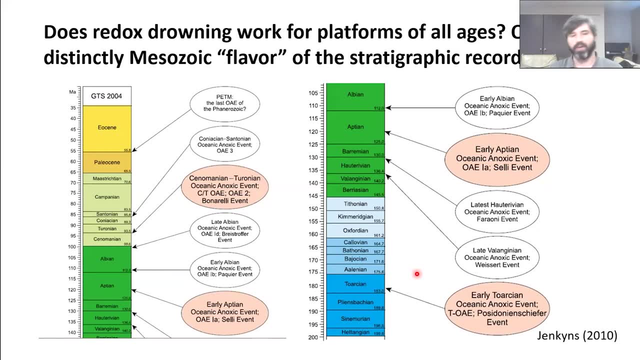 carbonate platforms. a lot of it's in coccoliths. And so then there's this evolutionary question of: well, wait a minute, you know when? when did coccoliths first appear? They actually didn't appear, you know, at the, you know, advent of animal life. in the latest Precambrian, They actually 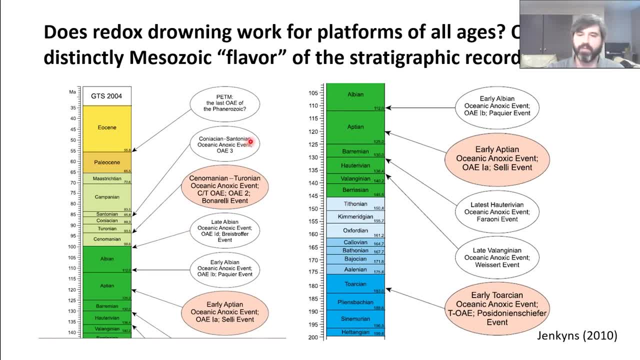 appear about halfway through the Phanerozoic, and this is something that people have picked on quite a bit, And this is a review paper from Hugh Jenkins Where he's talking about ocean anoxic events and he kind of highlights the four major ones of the 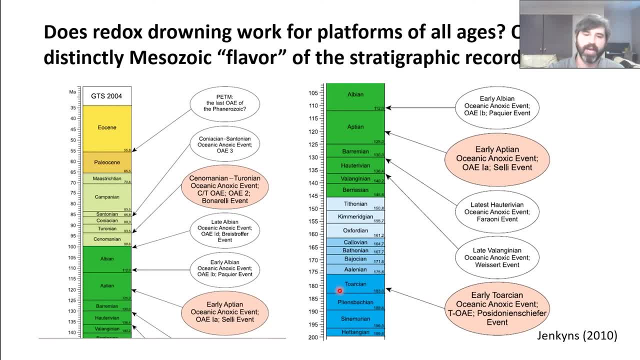 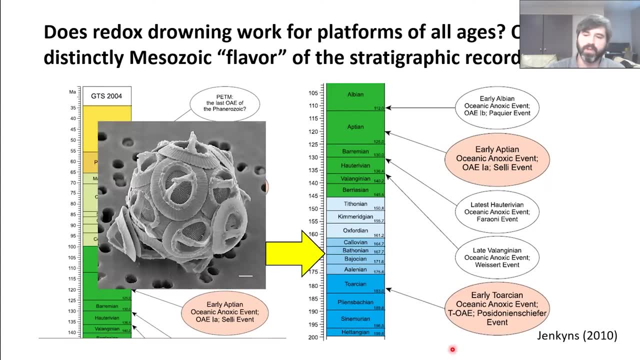 the Phanerozoic, which are the early Toartian, the early Aptian, OAE1a, there's another 1b event and there's OAE2.. And of these four events, only the early Toartian event is associated with a. 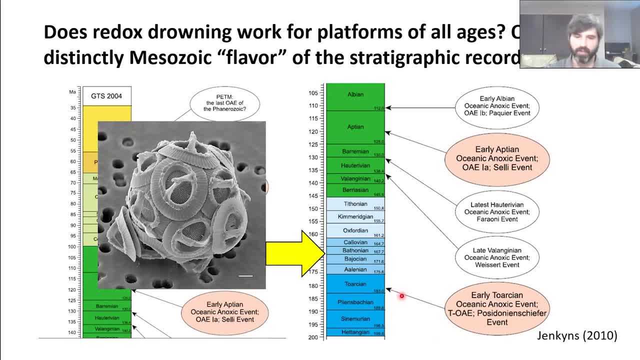 with a mass extinction and a large amount of biotic turnover, And people have really harped on this that you know these other ocean anoxic events are. I mean, they're really big disturbances of the earth system, but there's something about the ocean anoxic event that's really important to us, But there's 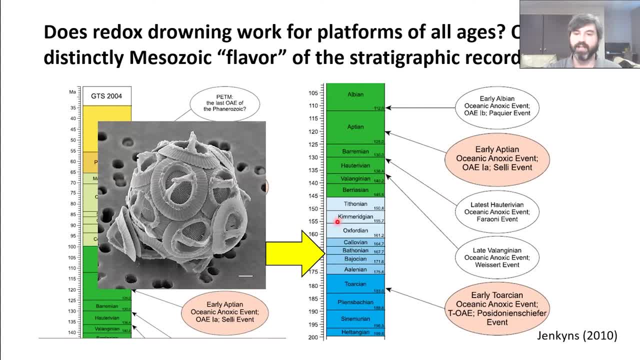 something about the ocean anoxic event that's really important to us, But there's something about the different about them. You know, the biotic change is is less and people pointed to these cocalists and said actually the appearance of these cocalists sometimes, or the spread of these cocalists during 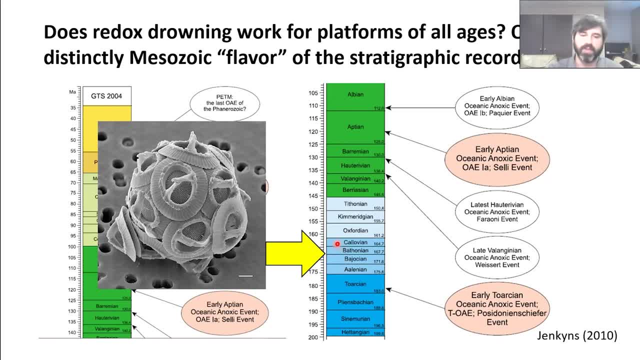 the mid-Messozoic marks a fundamental difference between the way the earth handles these disturbances, between the early Mesozoic and Paleozoic and then the kind of later Mesozoic and Cenozoic. And so from the perspective of what we're proposing here, you know, I would ask myself and I 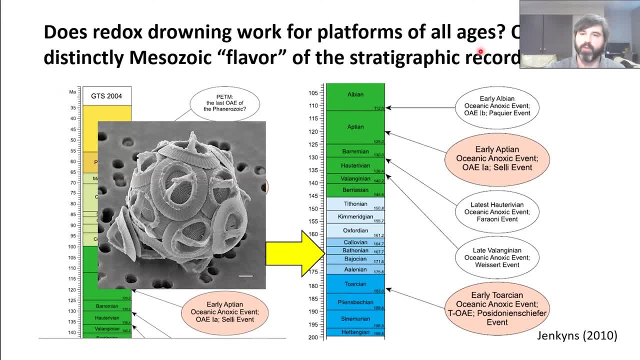 still ask myself: does redox drowning work for platforms of all ages? You know, do I want to go to the Devonian and use this for a Kelwassert event or something like that? Or is what we've outlined really a distinctly Mesozoic flavor of stratigraphic packaging that that is only? 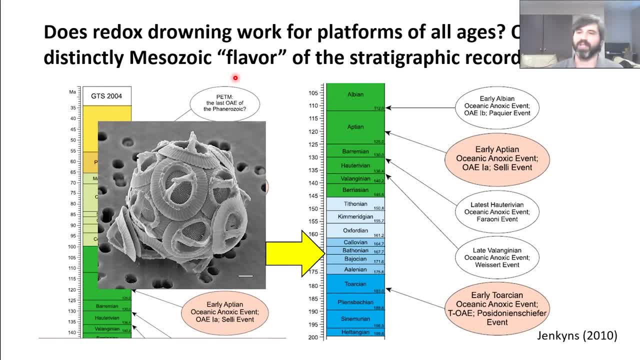 really valid for for like a short period of earth history and helps explain some of the differences between events that that nominally share the same trigger, which is this volcanism, but seem to be expressed differently within the the rock record. And that is all I have for now, and I'm 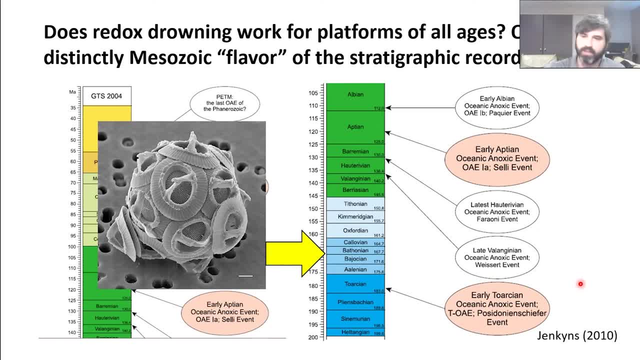 happy to to take questions, Kelly, if there's any questions. Thanks for a really cool talk, Ben Y'all. if you want to put questions in the chat or if you would like to unmute yourselves, just go for it. Hey, Ben Tony here. This is great, great talk. Hey Got a question for you, All right. 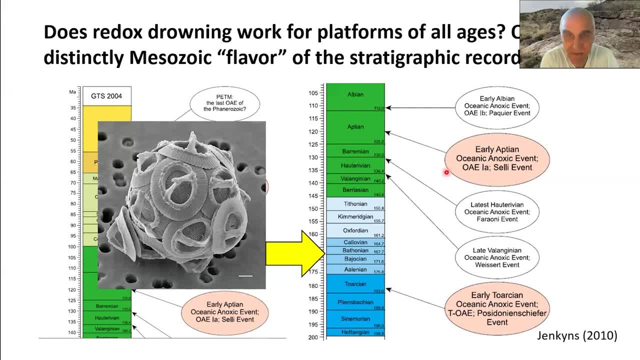 So with the um, I was trying to think with with your box model, like the non-synchronous um drowning of the carbonate platforms, is that? I mean, is that an indication that it's just not like the ocean's not well mixed with respect to uh alkalinity? 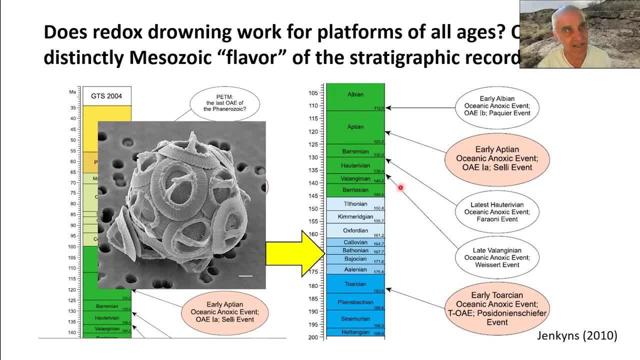 And do you think you can, or is it just is there, is it isn't not just like one event that kicks off drowning, You know, are there multiple events. I think your, uh, your box model approach could kind of highlight, at least identify, like what you think, the key processes. 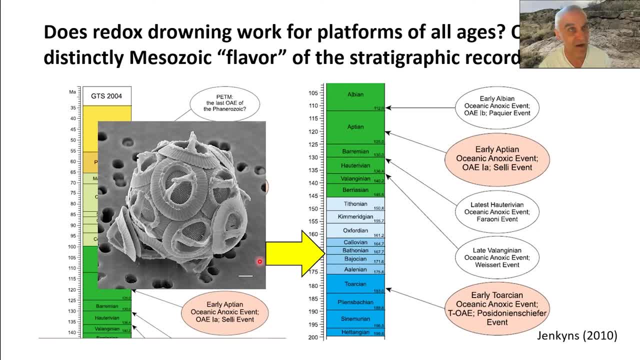 and then get that. and what's the time frame difference? you know, is it like a hundred thousand years or like two million year difference between these uh platform drawings around the world? It's a good question. So let me see if I can uh find a, find a. 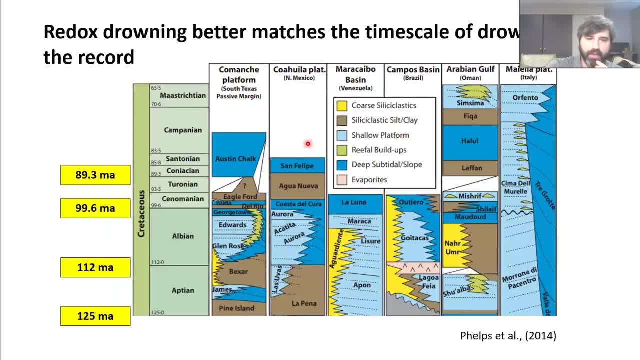 relevant slide here. uh, real quick, so yeah. so tony's question is about the time scale of these drownings and the differences between different regions of the world, and i i kind of harped on the idea that, like the, the carbon system in uh sea water tends to be. 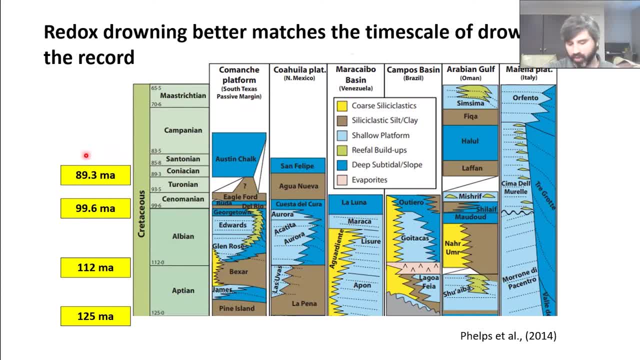 relatively well mixed, and and that a disturbance to the atmosphere will percolate into the ocean very quickly. um, one thing that i would point out is that in in the modern ocean, uh, there's differences in the depth between the carbonate compensation depth uh, between, like the pacific. 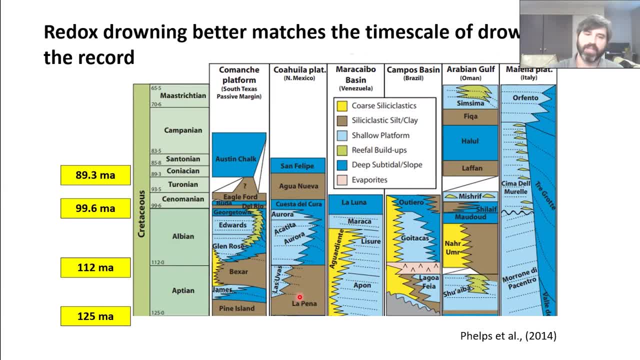 and the atlantic, and- and i think that's actually indicative of what we're talking about here- because the differences in those are not going to be related to pressure temperature gradients like i don't think those make that much of a difference. they're really going to be. 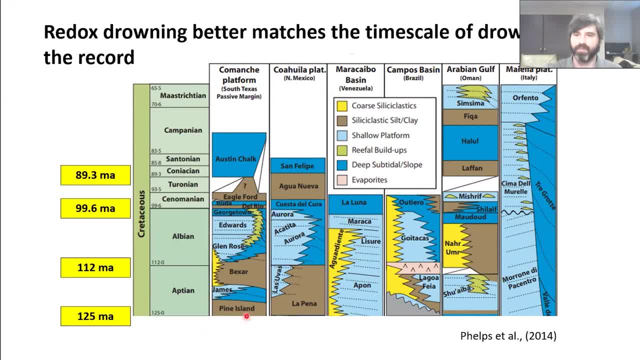 related to the organic matter flux and you know like how you know organic matter is being respired um and again, remember that that um aerobic respiration is is bad for carbonates. you know it'll either if, if you're super saturated, it'll lead to slower. 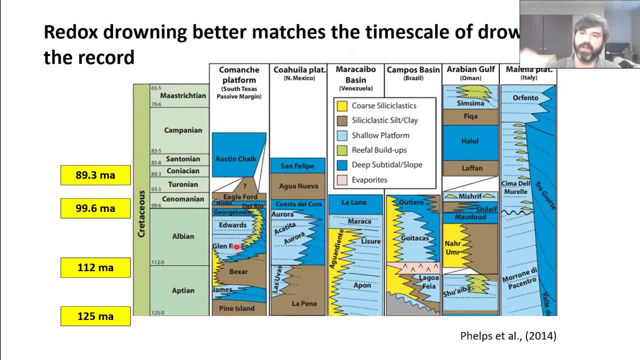 rates, and if you're under saturated it'll lead to faster dissolution rates. so that i think this um some chemical oceanography research that suggests that the depth of that ccd in different ocean basins is related to the organic matter flux and how organic matter is being respired, and so i would 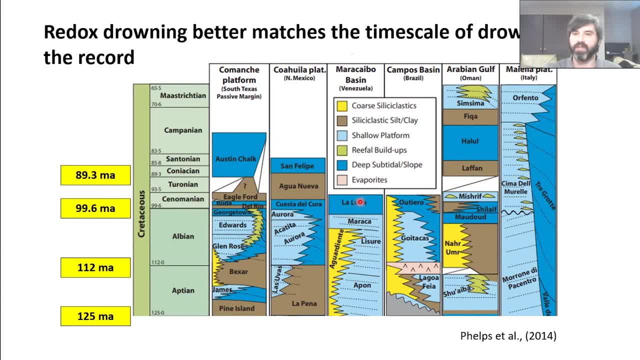 consider this kind of an extension of that. you know, saying that you know, even in our modern ocean we're not going to be able to see the difference between carbonate and carbonate dissolution with depth, and all we're doing is we're playing, we're kind of playing based on that and and i i don't see any reason why those 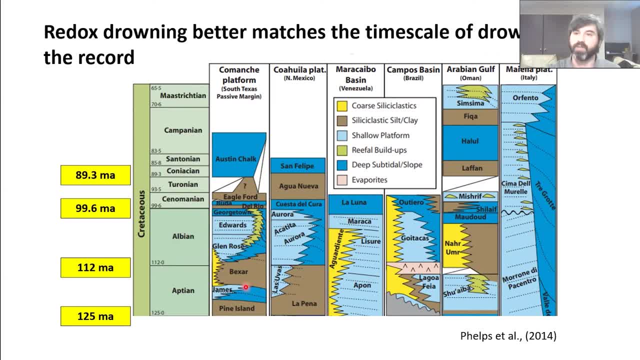 kind of those differences would disappear when we start adding different metabolisms. is that? is that answer enough for your question? yeah, no, that's good. i like that idea that sort of: are the mud rocks chasing the carbonates? are the carbonates chasing the mud rocks? yeah, i. i will add one other thing of interest, and it's something that's just not touched on in this. 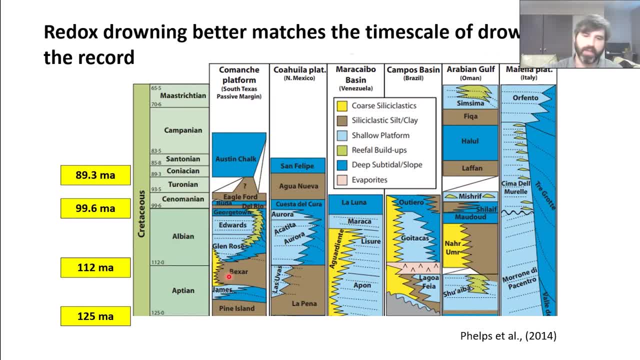 talk at all and i'm sure some people are interested in it. you know there's plenty of drowning events during the cretaceous that don't seem to line up with a ocean anoxic event, and and i and i also think about, you know, like uh ahmed al-nawi's phd and some of the work that 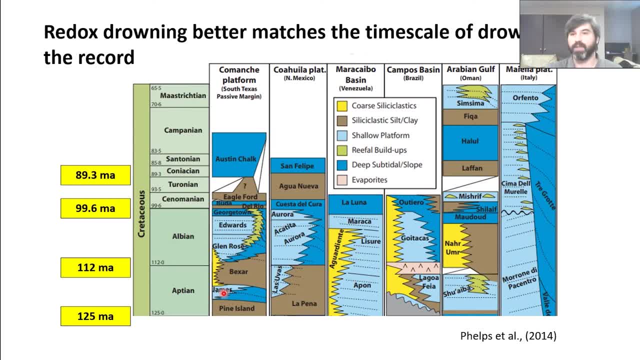 you and you and bob had done with him, where for oae2 it's like the best, the best organic matter and the highest trace elements enrichments are actually below the ocean and oxygen, and so, like i, i still struggle with that. you know the, the, the match between the geochemical and the physical. 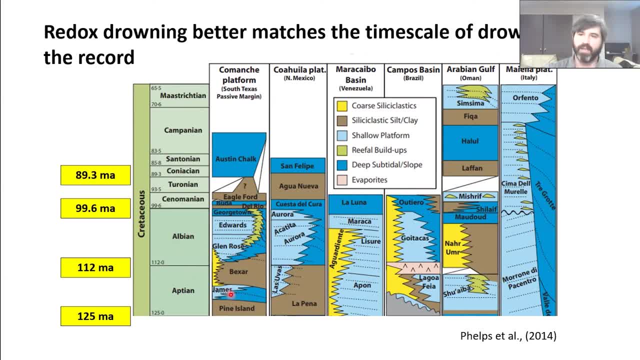 records is rarely as clean as we would like it to be, and so i don't think this model totally solves that, but it at least tries to grapple with that saying like you know, how can we make spatial and temporal differences, you know, between these different ocean basins? that that give you some. 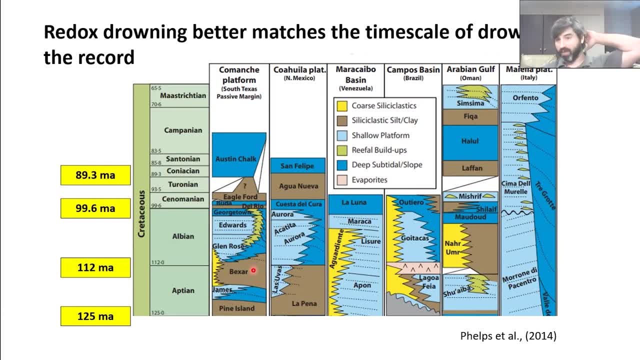 wiggle room for how the stratigraphic record and the geochemical records are going to match up. i think richard's question in the chat box goes right into that. yeah, so uh, richard den says the drowning of the buta platform occurred around 97.5 million years. 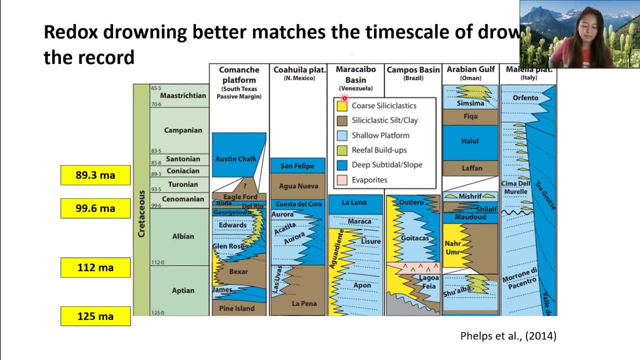 uh, several million years prior to oae2? yeah, that's a great observation. um, so yeah, a lot of the carbonates in the gulf coast drown, you know, way before oe2. it's possible they're co, they're coincident with this oae1d. 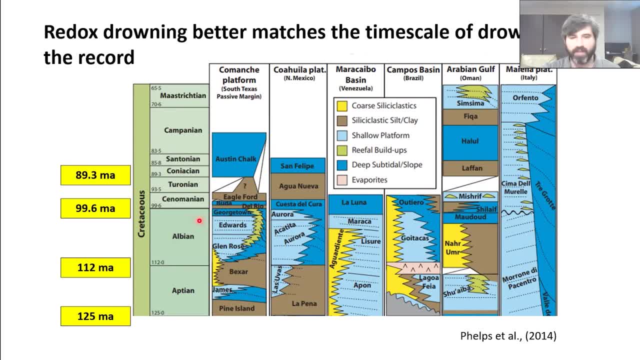 but i, i it doesn't really matter. it's a very valid concern, which is: oae 1d is a smaller event and even if you were to correlate it, you still have this problem of: okay, well, why isn't oae1d knocking out carbonate platforms in italy? and then what is it? 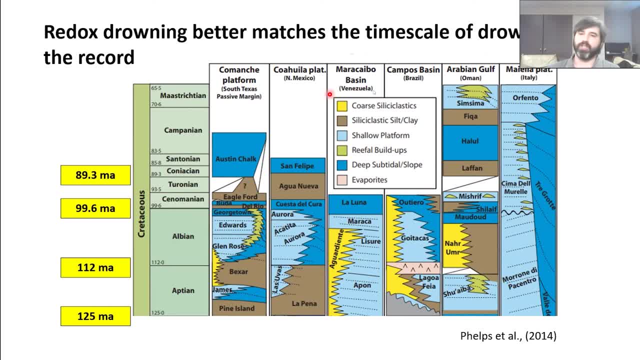 even mean if you have an ocean intoxic event which is, like, usually defined as a global phenomenon. what does it mean when you have, like oae1d or oa3 or some of these oaes that people argue about whether they're regionally expressed or not? um, and again, i do think that there's a little bit. 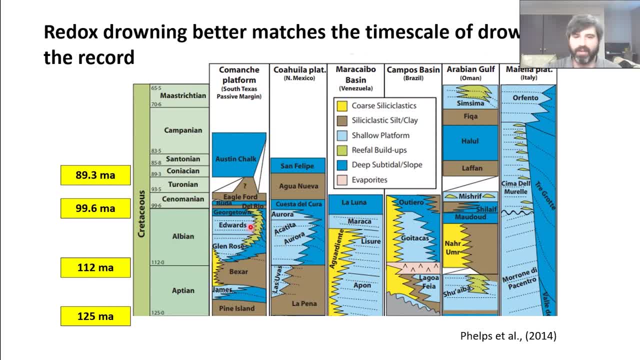 of flexibility within this model, which is, like you know, it actually doesn't have to be an ocean anoxic event, and one of the things that showed up in this, the biomarker studies was like, yeah, there's 什麼大的改进, cam PDF contterniという企业的存位. fascia studies was like, yeah, there's a change in biomarker models. and the car was a little. 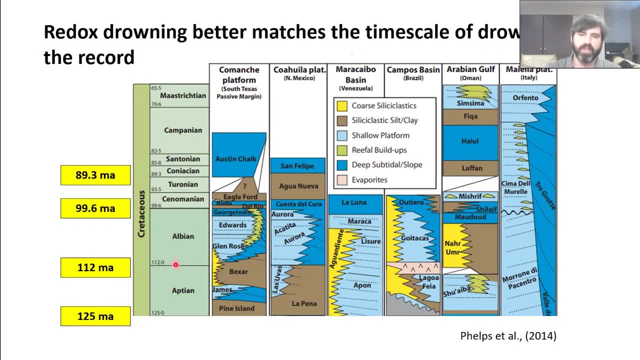 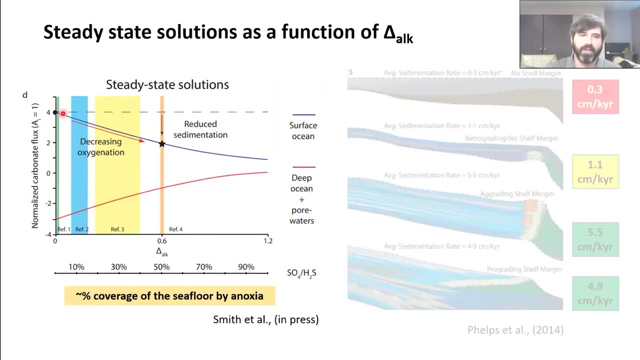 associated with OEEs. There's also sometimes evidence of these biomarkers showing up just in regular Cretaceous sediments above or below the event, And so one possibility that I'll throw out there, with very little to substantiate it, is that in these greenhouse worlds, when you have 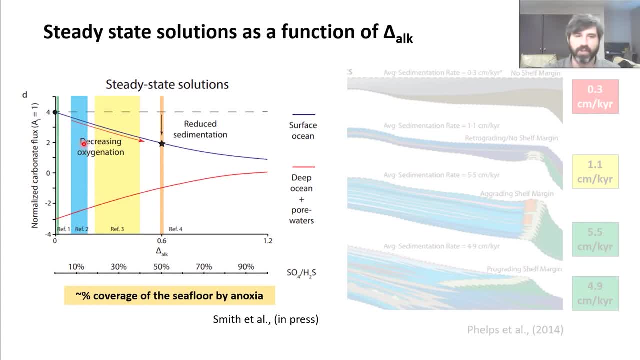 kind of slow ocean circulation. you don't have ice caps to drive ocean circulation. there may just be pockets of anoxic water hanging around- They don't all need to be correlated with these ocean anoxic events- And then so you might just be kind of sliding up and down this curve as those 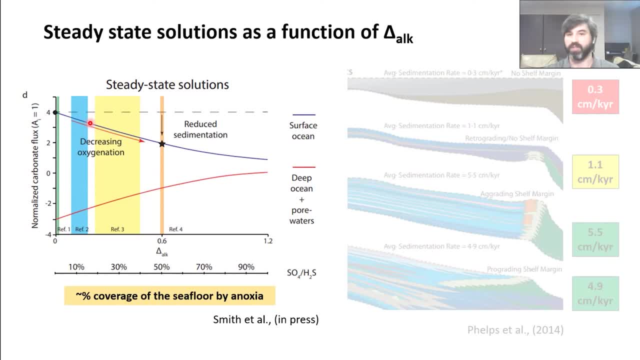 pockets kind of appear and disappear and there's other processes that are changing circulation, And so, yeah, I do appreciate this idea that it's probably harmful to try to, like, use a hammer to hammer everything and make it fit into an ocean anoxic event when there's clearly 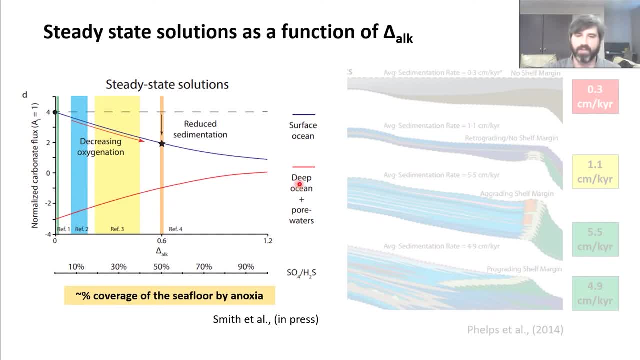 other processes going on that also drive circulation. And so yeah, again, I would say I'd be interested in the biomarkers in the Buda, you know. are there biomarkers associated with changing microbial metabolisms? If so, great. If not, that's a sign. 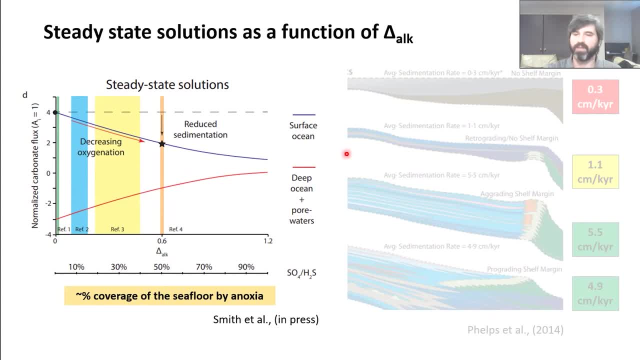 that it's time to move on And this is not the model you want to be applying. To follow up on that, he says, we found that the concretionary layers in the Eagleford were preferentially bioturbated versus the organic layers. And so, yeah, I would say, yeah, I would. 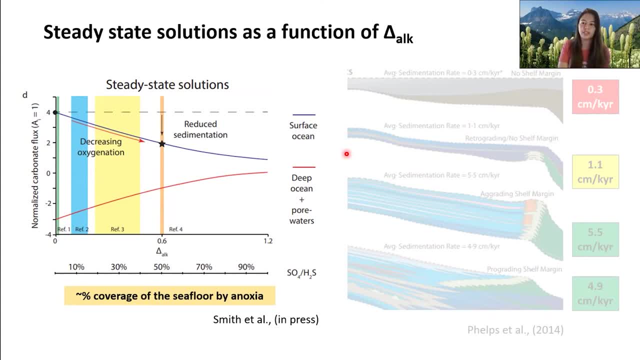 be interested in the organic rich layers, which we also attribute to microbial related changes in sediment alkalinity changes. So I think you're on the right track, Right on. Okay, cool, I would love to talk to you about that more. If you have time, I'd love to. 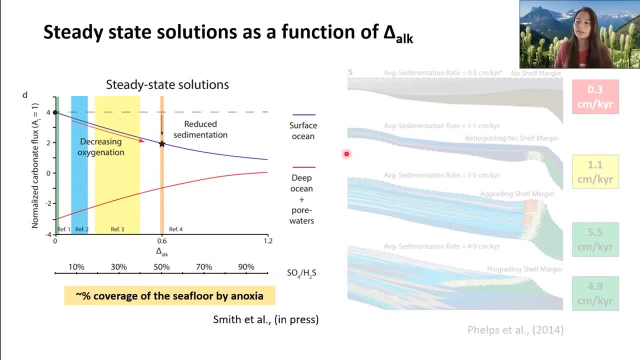 meet with you after the talk. Yeah, there are still a couple of slots right after the talk available, So okay. so going back to a question from Ali Abraham Libraham. sorry, They say, if the oceans recover quickly from acidification, what mechanism explains prolonged anoxia or ocean? 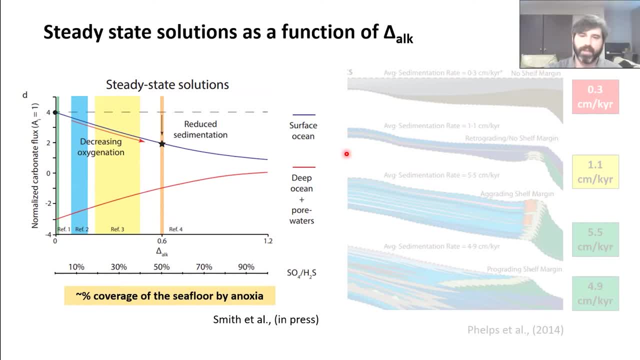 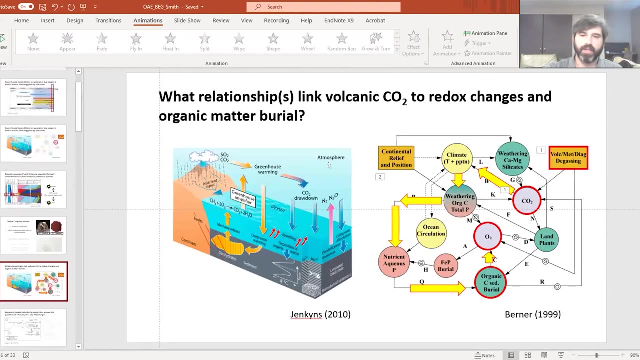 acidification? Yeah, that's a good question. My understanding is that most of the anoxia- let me see if I can go back here- Most of the anoxia is going to follow the same route as organic matter. So it's going to follow the same route as organic matter. So it's going to. 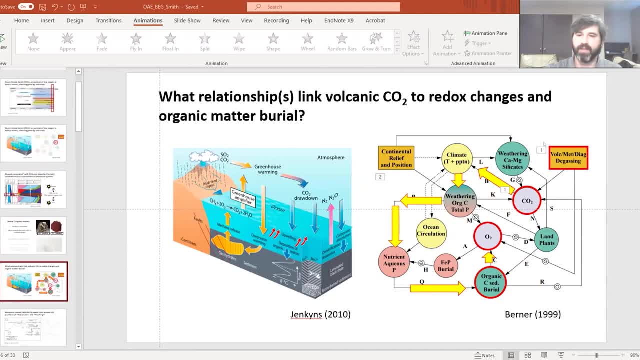 follow the same route as organic matter. So it's going to follow the same route as organic matter. It's going to follow this timescale of weathering feedbacks. So the CO2 triggers this weathering feedback that increases the delivery of nutrients to the ocean. So it's going to follow this arm. 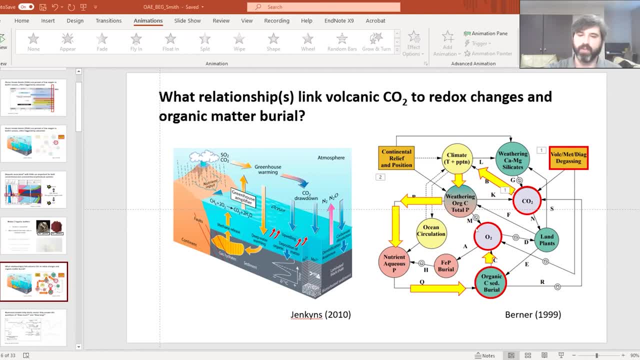 right here, which goes with the timescale of organic matter enrichment and oxygen budgets. What I'm less good at is that there are characteristic timescales associated with all of Earth's geochemical cycles, And I'm told that the oxygen and redox budgets tend to evolve on million-year timescales. And then the carbon 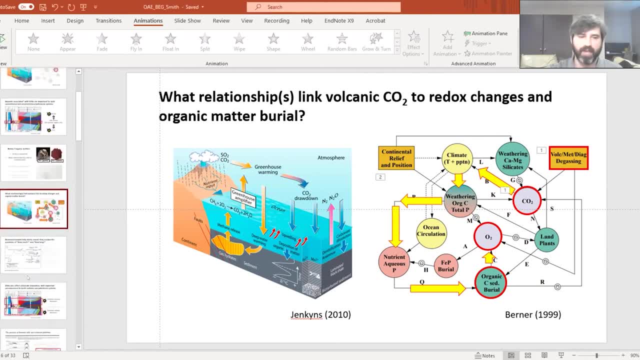 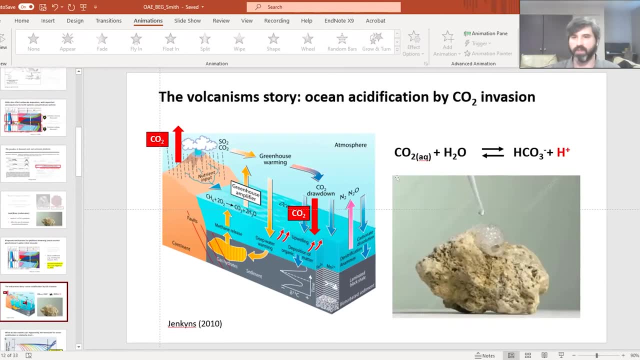 budgets, like if I have a carbon budget that doesn't interact with redox, like this ocean acidification story. those tend to evolve on very short timescales, And so that's a part of the interdisciplinary aspect. that's just a little outside my